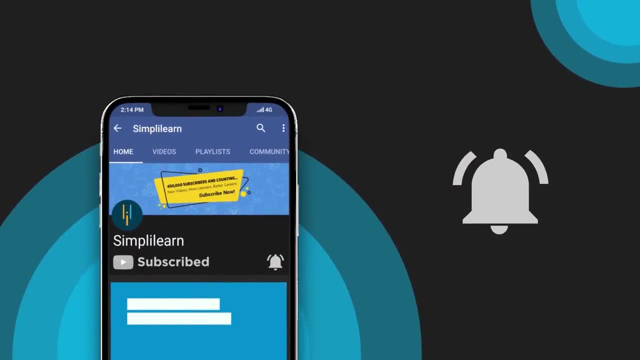 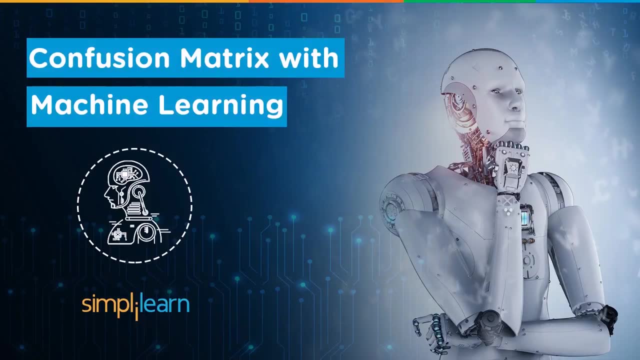 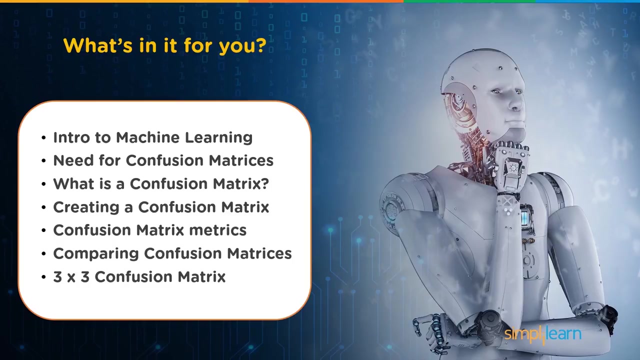 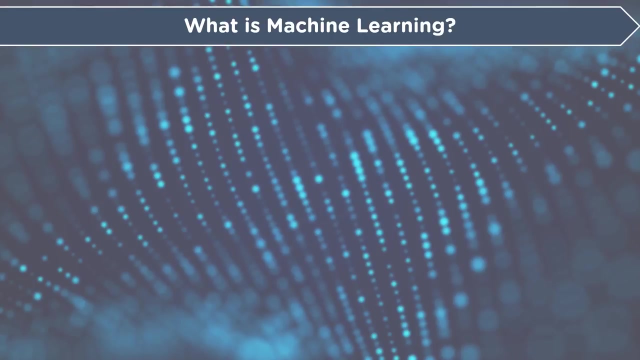 Confusion Matrix with Machine Learning. What's in it for you? Intro to Machine Learning: Need for Confusion Matrixes. What is Confusion Matrix? Creating a Confusion Matrix, Confusion Matrix metrics Comparing Confusion Matrixes Three by three. Confusion Matrix: What is Machine? 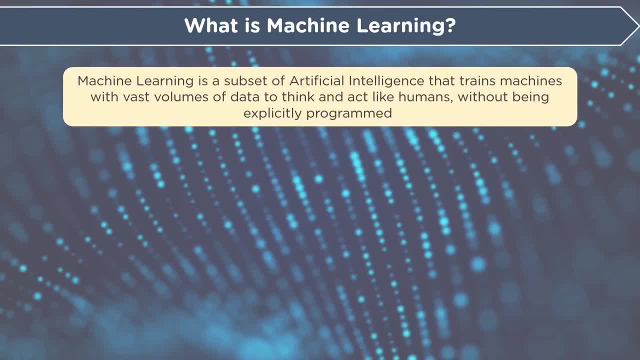 Learning. Ah, so we're going to jump into Machine Learning first, because you have to have that overview. Confusion Matrix is about understanding the results of your Machine Learning and validating it. Machine Learning is a subset of artificial intelligence that trains machines with vast volumes of data to think and act like humans Without being 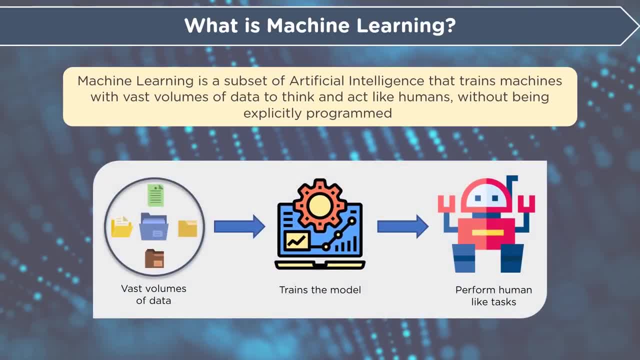 explicitly programmed. So you see, here we have a vast volumes of data that come in. You have a trains the model. So we have our model, kind of like a black box, And then it performs some human-like task. In today's Machine Learning that usually has to do with 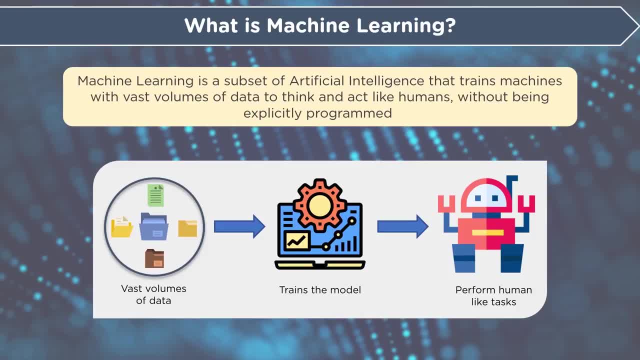 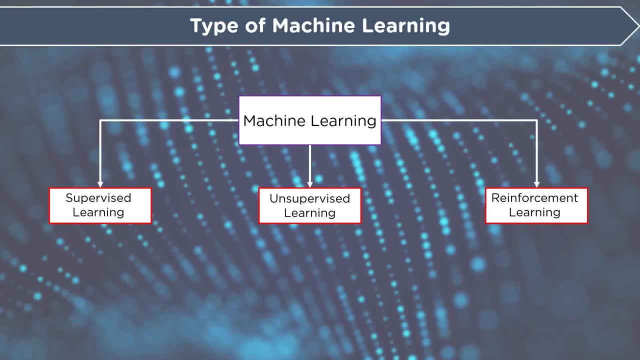 a lot of prediction of what the future is, or predict the best option to go forward on. So in the type of Machine Learning, there are three major categories, And so we have our Supervised Learning, Unsupervised Learning, Reinforcement Learning. 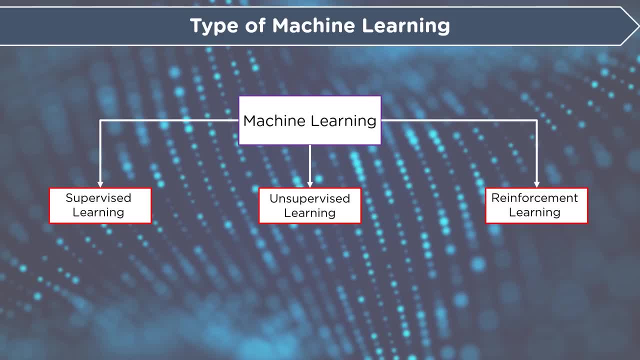 Then we talk about Supervised Learning. Think about it. you already know the answer. This is: you have a huge amount of data, you already know what you want out of it, and so we're going to train the model to find that data Unsupervised. 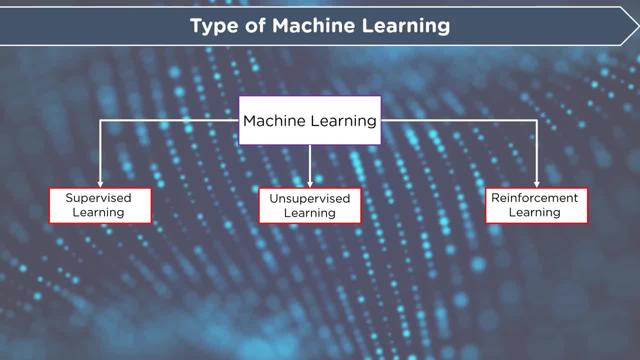 Learning means we're just looking for stuff that matches. We don't know what goes together. we don't know what's going to fit together, So it doesn't really have an answer. It just says, hey, some of these things fit together. 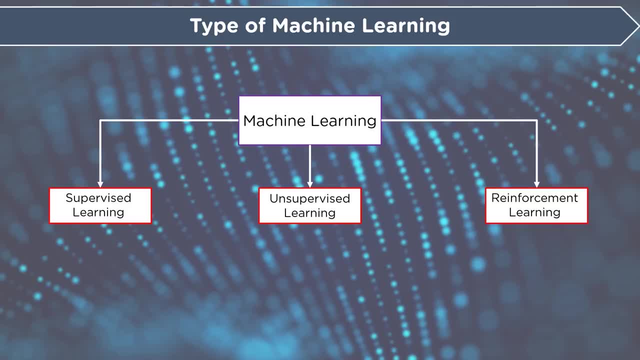 Let's see if we can find them. And then reinforcement learning is- you don't know the answer until it happens. So you can think of this as you do something and you get a reward, And so there's a. reinforced learning is like the cutting edge right now, So there's a lot of 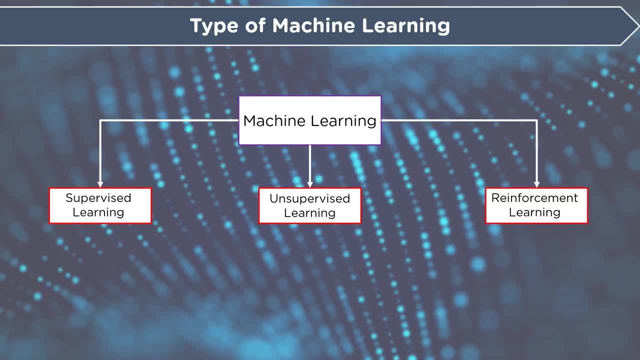 Now we talk about supervised learning. think about it. you already know the answer. Uh, so this is: you have a huge amount of data. You already know what you want out of it, what's going to fit together. so it doesn't really have an answer. it just says, hey, some of these. 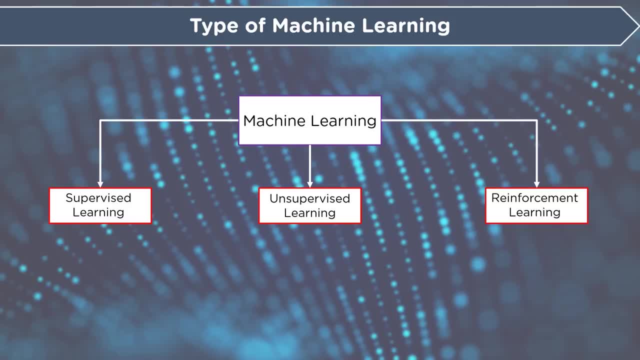 things fit together. let's see if we can find them. and then reinforcement learning is- you don't know the answer until it happens, so you can think of this as you do something and you get a reward, and so there's a. reinforced learning is like the cutting edge right now, so there's a lot of. 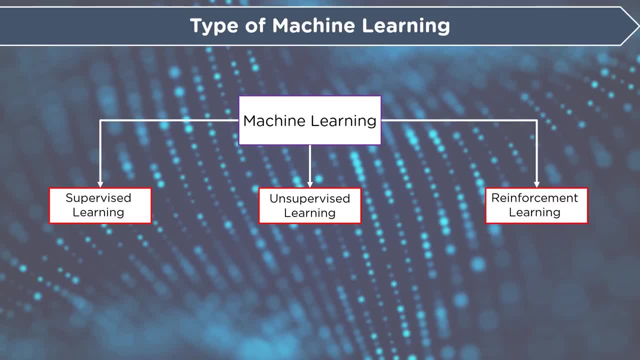 work being done in that, as in all of these, but that would really be the one that is still they're trying to figure out. and when we talk about supervised learning, we have regression, and when you see the word regression, think numbers, use these float values and classification. 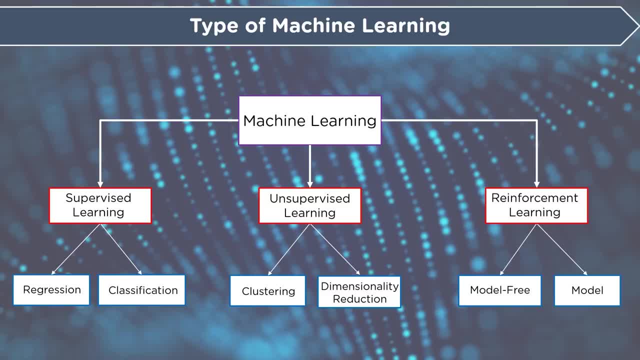 classification is true, false, yes, no, this is a dog, that is a cat. when you're doing pictures and things like that, and then when you have unsupervised learning, there's clustering. some of these things fit together and we cluster colors together. we cluster them by both location and color in an image. it might be you are clustering different measurements, that 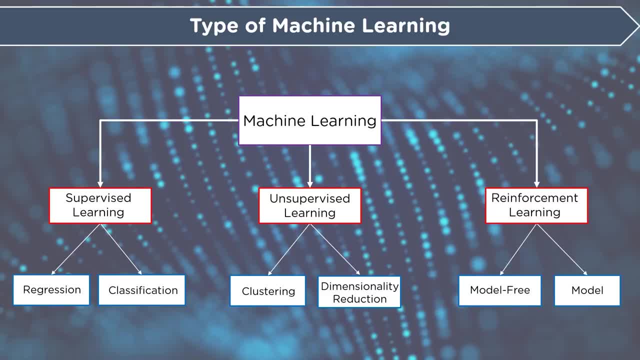 kind of fit together somehow, and then dimensionality reduction. so this is, the more simplified we can make, it the better. so each classification is based on removing the chaos as it is in the thing and bringing more similarity to each area, and then, with the reinforcement learning, there's what they. 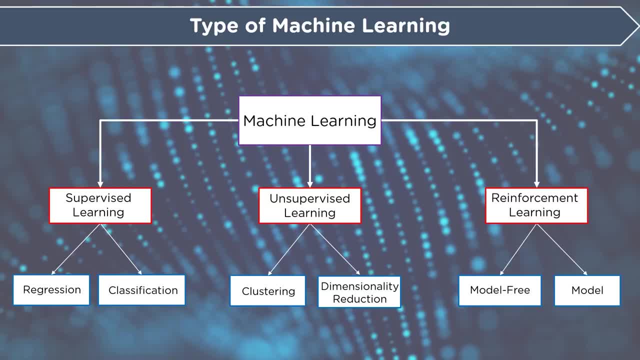 call model free. model free is you're not actually training a model. this is kind of like you build a chart: this is what happened, this is what the this is what went into it, sort of thing. and then there's also model building. so you train the model as it goes. so we're going to drill down to what is classification I touched. 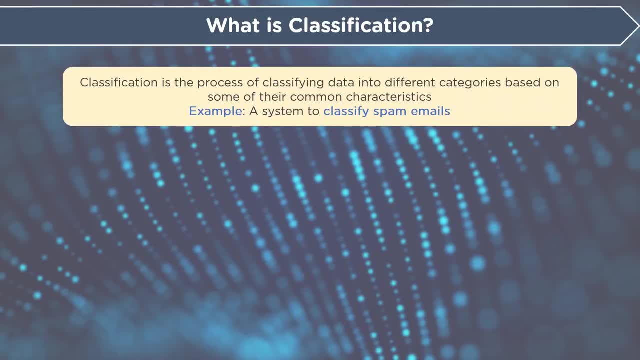 upon all those different aspects. that classification is the yes, no, you're classifying it as something, and the reason they spend a lot of time on classifying is because they don't know what classification is, because one of the easier ones to understand, it's a little easier to track, it's a 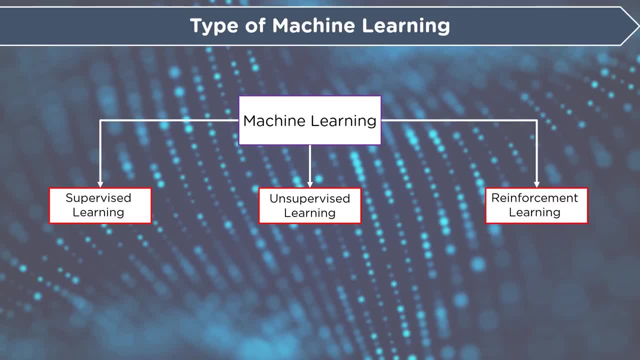 work being done in that, as in all of these, but that would really be the one that is still they're trying to figure out. And when we talk about supervised learning, we have regression. And when you see the word regression, think numbers. Usually it's float values and classification. 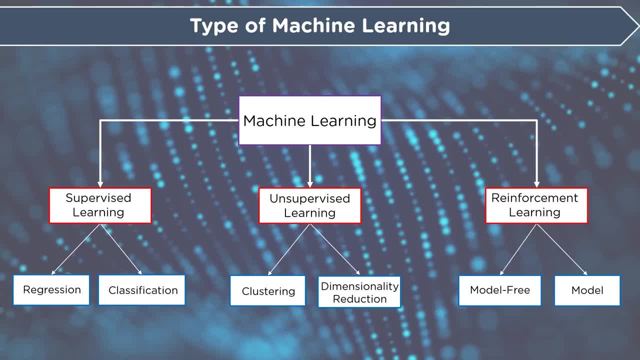 Classification is true, false, yes, no, This is a dog, That is a cat. when you're doing pictures and things like that, And then when you have unsupervised learning, there's clustering. Some of these things fit together and we cluster colors together. Can we cluster them? 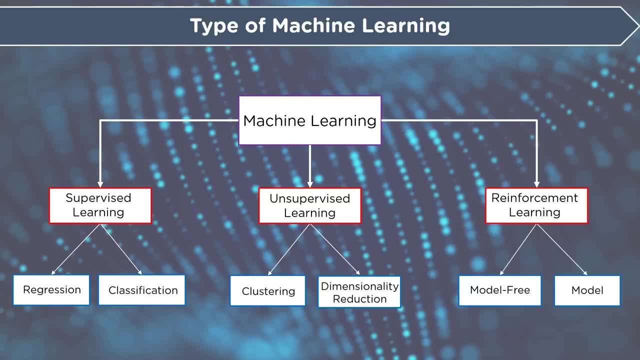 By both location and color In an image. it might be you are clustering different measurements that kind of fit together somehow, And then dimensionality reduction. So this is, the more simplified we can make it, the better. So each classification is based on removing. 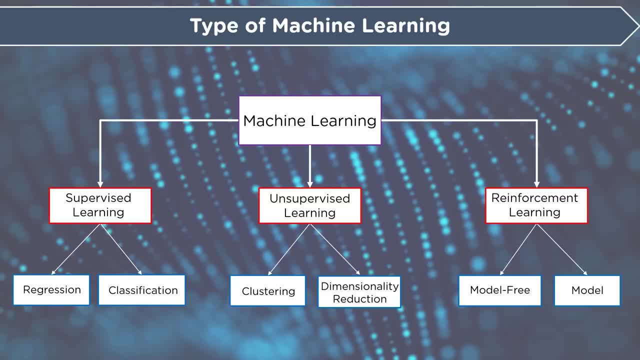 the chaos as it is in the thing and bringing more similarity to each area. And then, with the reinforcement learning, there's what they call model-free. Model-free is you're not actually training a model. This is kind of like you build a chart. 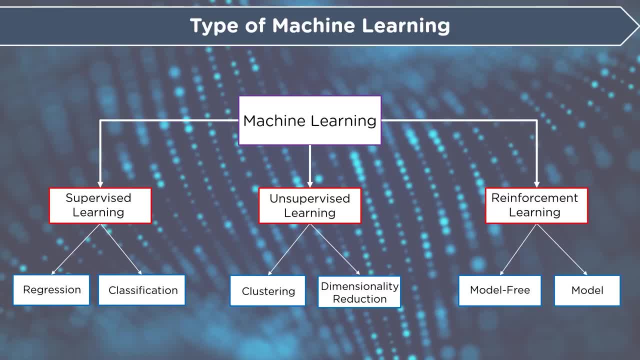 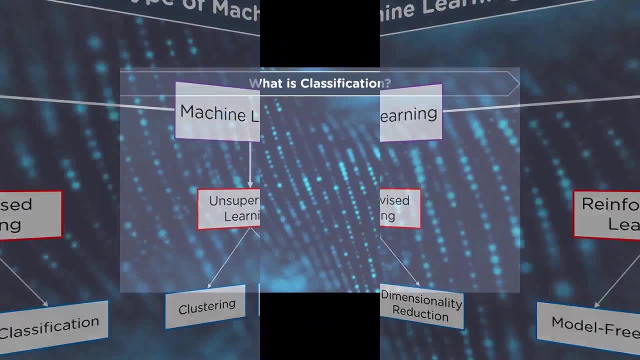 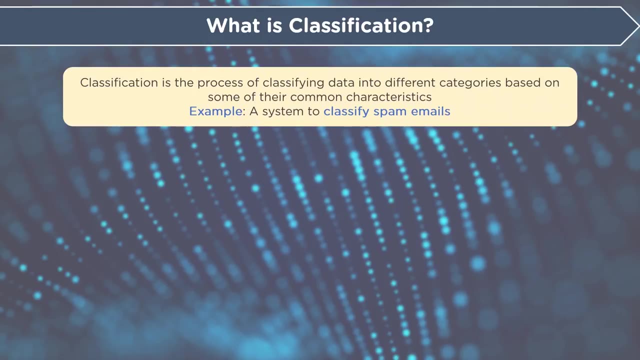 This is what happened, This is what went into it, sort of thing. And then there's also model building. So you train the model as it goes. So we're going to drill down to what is classification. I touched upon all those different aspects. that classification is the yes, no. You're classifying. 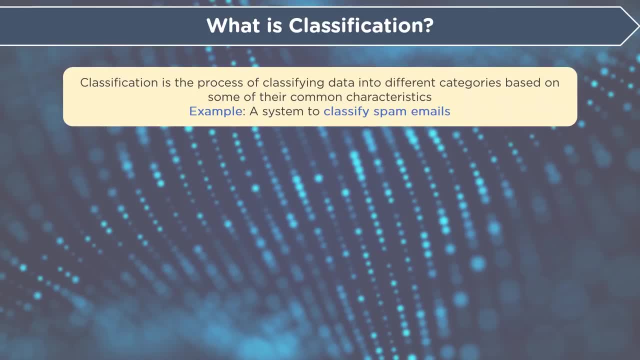 it as something, And the reason they spend a lot of time on classification is because they're classifying it as one of the easier ones to understand. It's a little easier to track, It's a little easier to figure out the errors on it And when we're talking about a confusion matrix. 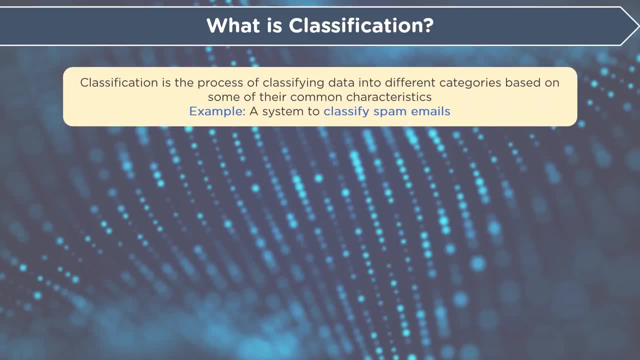 we're usually talking about classification, And I'll show you why here in a little bit. Classification is a process of classifying data into different categories based on some of their common characteristics. Example: a system classifying spam email, And you can see here. 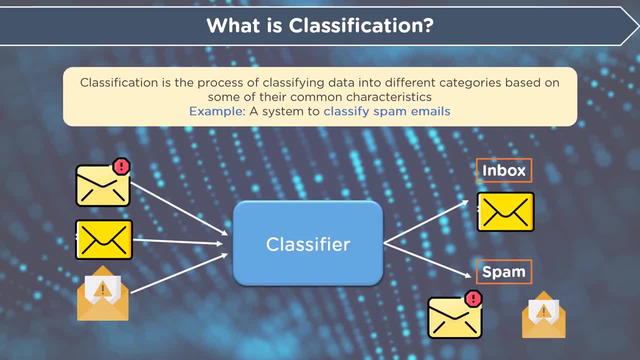 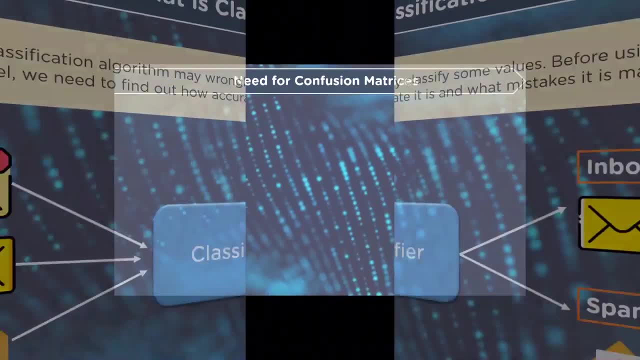 we have our email coming in. Some of them are spam, Some of them are not, And the classifier has to only say yes or no, It's spam or it's not spam. Need for confusion matrices. Classification models have multiple output categories. 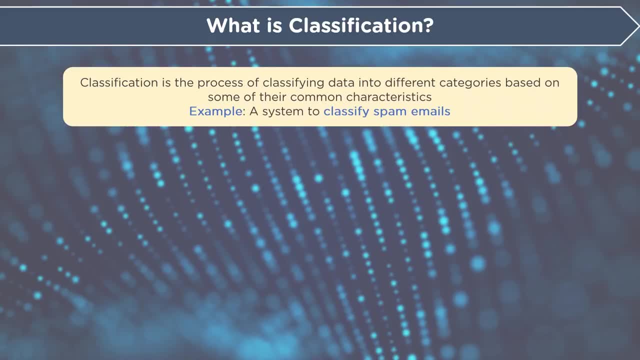 little easier to figure out the errors on it. and when we're talking about a confusion matrix, we're usually talking about classification, and I'll show you why here in a little bit. classification is a process of classifying data into different categories based on some of their common 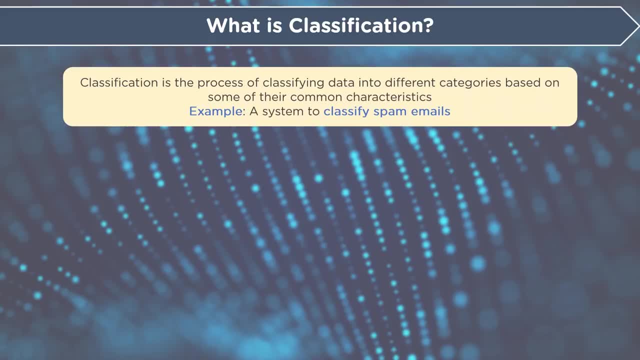 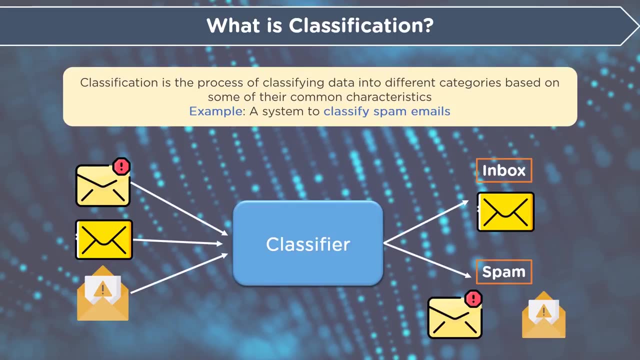 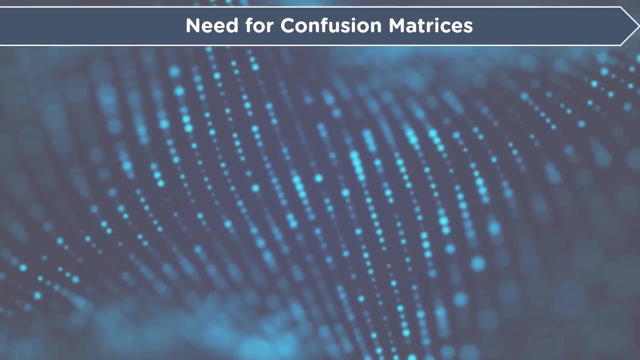 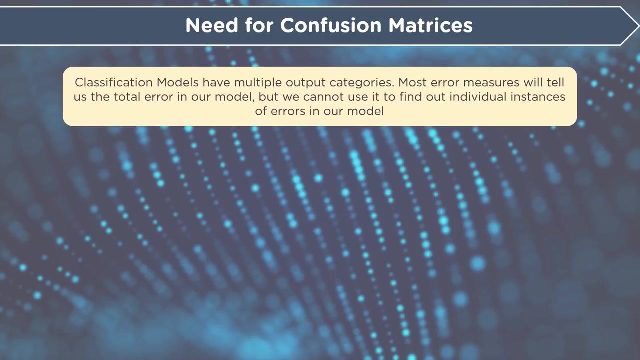 characteristics. example: a system classifying spam email and you can see. here we have our email coming in. some of them are spam, some of them are not, and the classifier has to only say yes or no, it's spam or it's not spam. need for confusion. matrices classification models have multiple output categories. most error measures will tell. 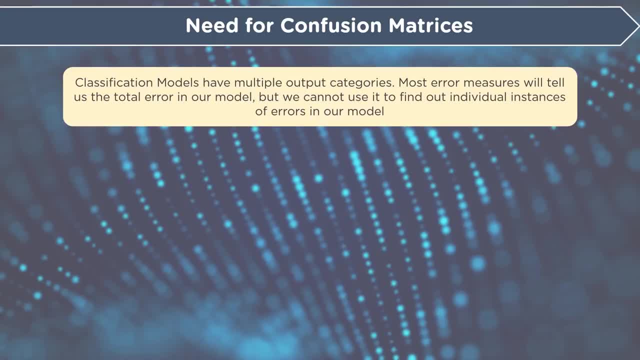 us the total error in our model, but we cannot use it to find out individual instances of errors in our models. so you have your input coming in, you have your classifier. it measures the error and it says: oh, 53 of these are correct. so you have your input coming in and you have your classifier and 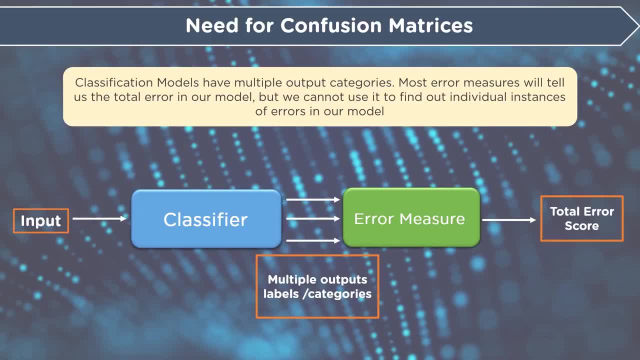 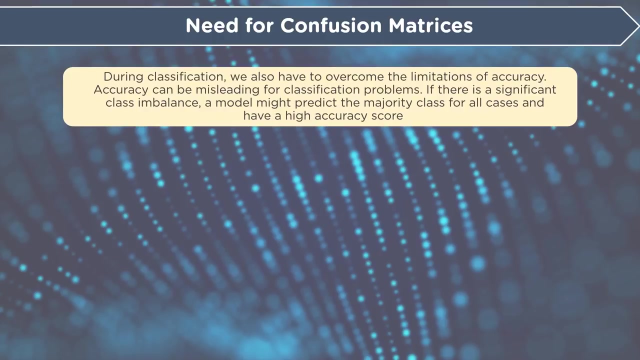 it says: oh, 53 of these are correct, but we don't know which 53% are correct. is it 53% correct on guessing on the spam? is it 23% guessing on spam and 27% guessing on what's not spam? this is where the confusion matrix comes in. so during the classification we also have to overcome the limitations of accuracy. accuracy can be misleading for classification problems if there is a significant class imbalance. 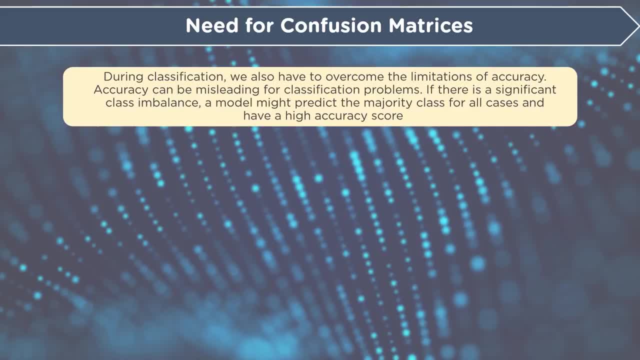 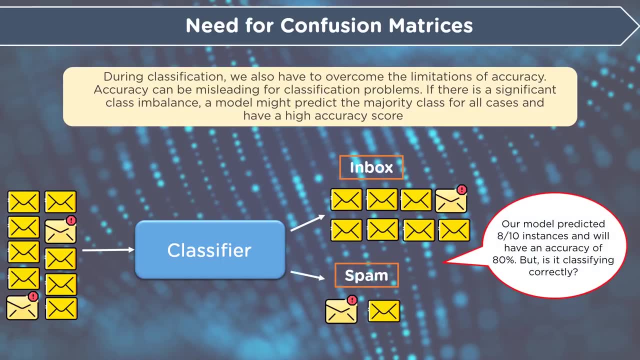 a model might predict the majority class for all cases and have a high accuracy score. and so you can see here: we have our email coming in and there's two spams. the classifier comes in and goes: hey, it only catches one of those spams and it misclassifies one that's not spam. 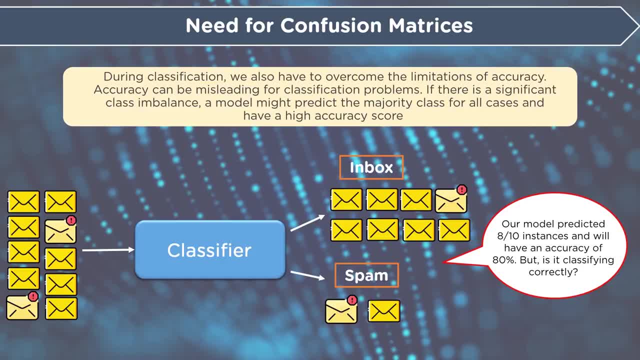 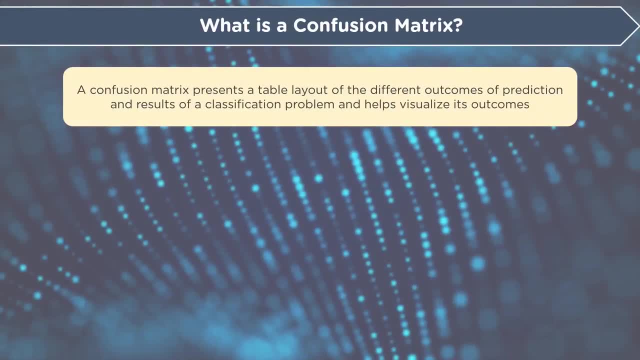 so our model predicted eight out of ten incidents and will have an accuracy of 80, but is it classifying correctly? a confusion matrix represents a table layout of the different outcomes of prediction and results of a classification problem and helps visualize its outcomes. and so you see, here we have our simple chart predicted. 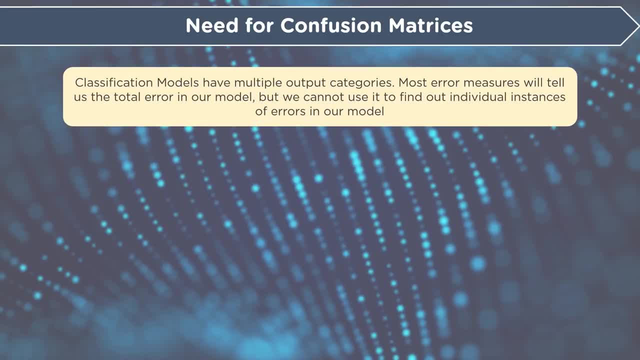 Most error measures will tell us the total error in our model, But we cannot use it to find out individual instances of errors in our models. So you have your input coming in, You have your classifier, It measures the error and it says: oh, 53 of these are correct. 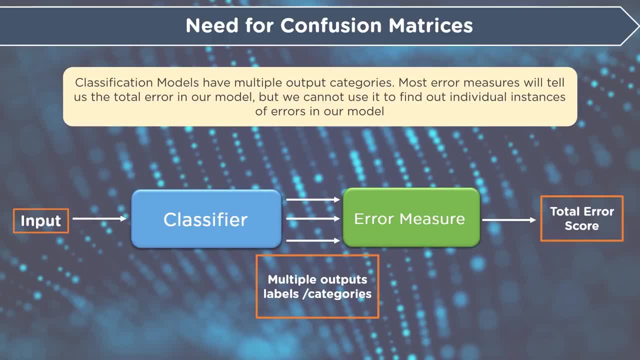 But we don't know which 53% are correct. Is it 53% correct on guessing on the spam? Is it 23% guessing on spam And 27% guessing on what's not spam? This is where the confusion matrix comes in. 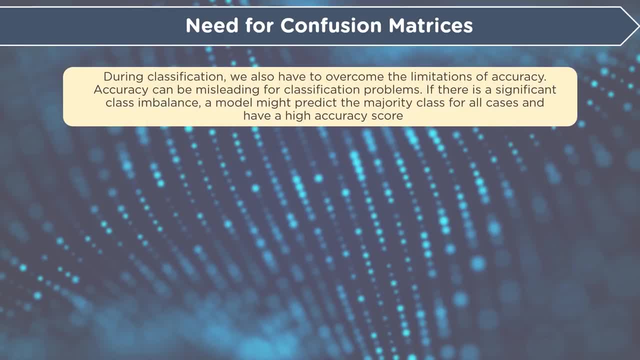 So during the classification we also have to overcome the limitations of accuracy. Accuracy can be misleading for classification problems. If there is a significant class imbalance, a model might predict the majority class for all cases and have a high accuracy score. And so you can see here. we have our email coming in and there's two spams. 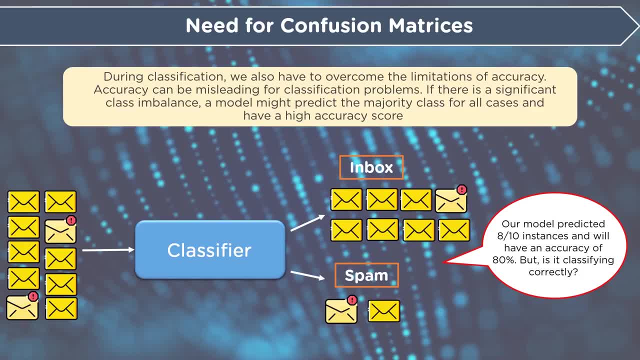 The classifier comes in and goes: hey, it only catches one of those spams and it misclassifies one that's not spam. So our model predicted eight out of 10 incidents and will have an accuracy of 80%. But is it classifying correctly? 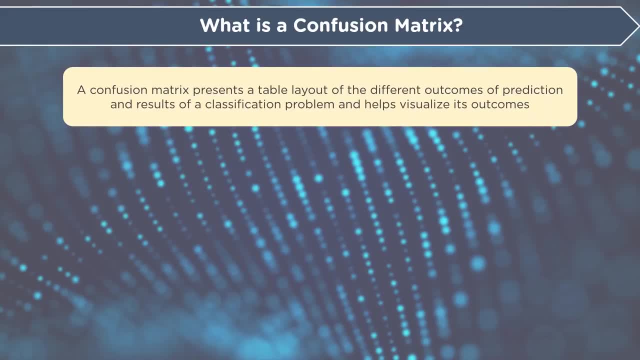 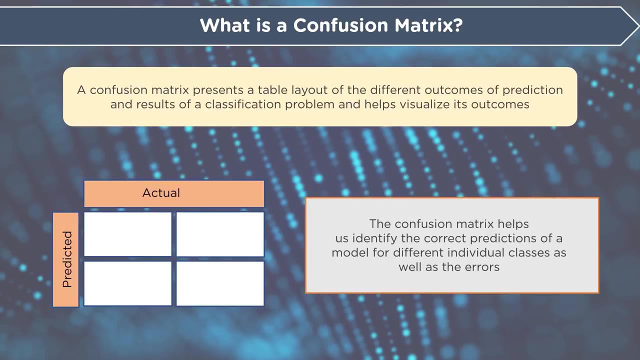 Confusion matrix represents a table layout of the different outcomes of prediction and results of a classification problem and helps visualize its outcomes. And so you see, here we have our simple chart, predicted and actual. The confusion matrix helps us identify the correct predictions of a model for different individual classes. 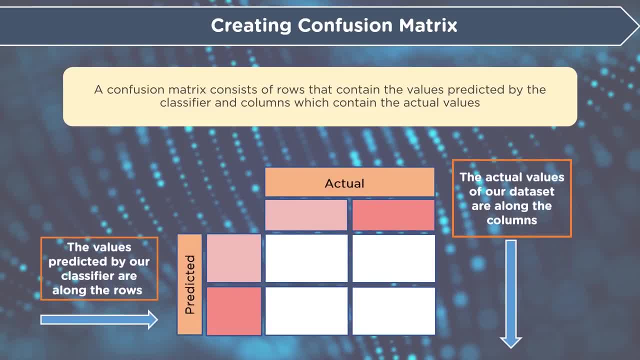 as well as the errors. So you'll see here that the values predicted by our classifier are along the rows. This is what we're going to guess. it is, or our model is guessing what. this is based on its training. So we've already trained. 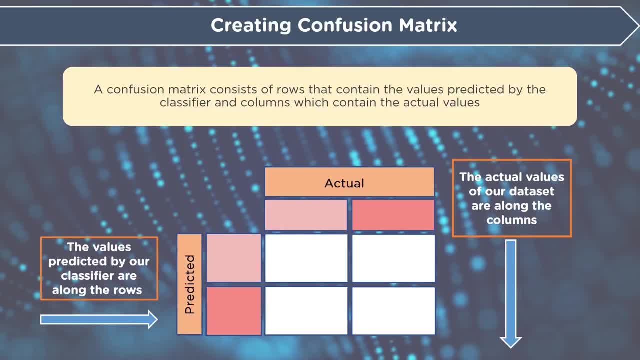 the model to guess whether it's spam or not spam or whatever it is you're working on, And then the actual values of our data set are along the columns. So this is the actual value. that's supposed to be. People who can speak English will. 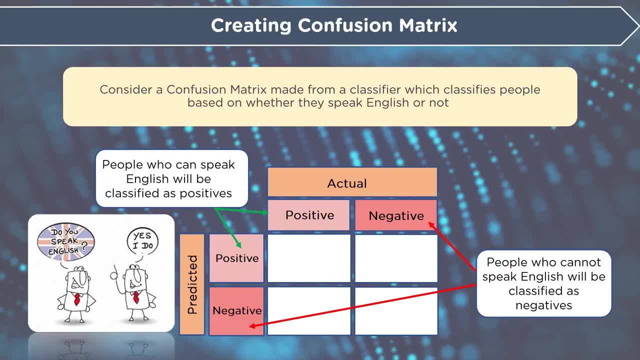 be classified as positives because they have a number zero or one. Do you speak English? Yes, no, And you could extend this that they might have. Do you speak French? Do you speak whatever language it is, And so you might have a whole lot of classifiers that you would look at each. 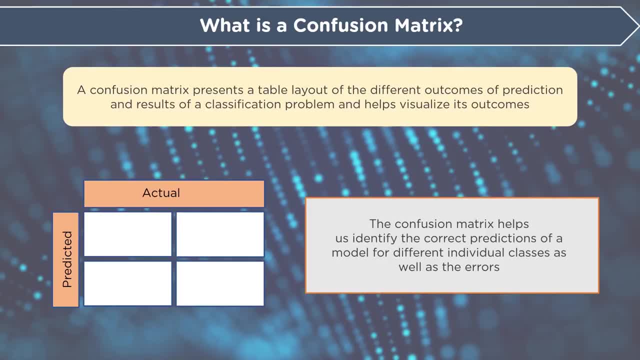 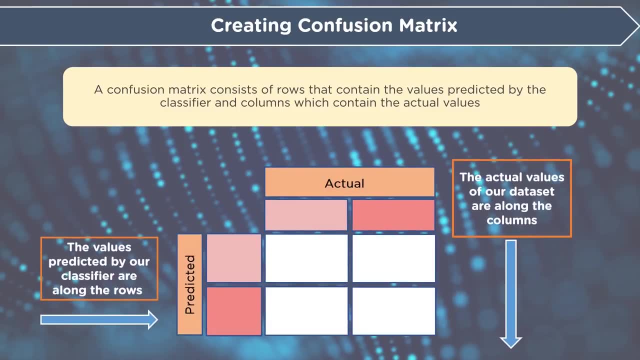 and actual. the confusion matrix helps us identify the correct predictions of a model for different individual classes, as well as the errors. so you'll see here that the values predicted by our classifier are along the rows. this is what we're going to guess. it is or our model is guessing. 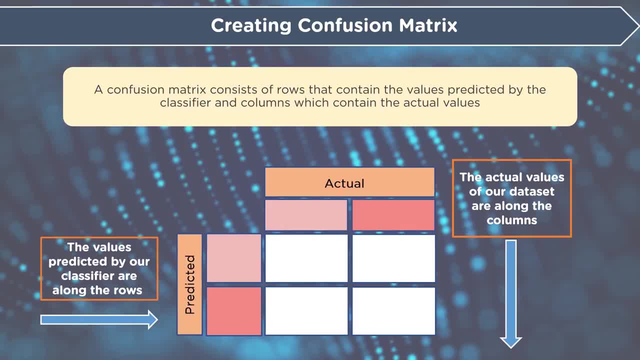 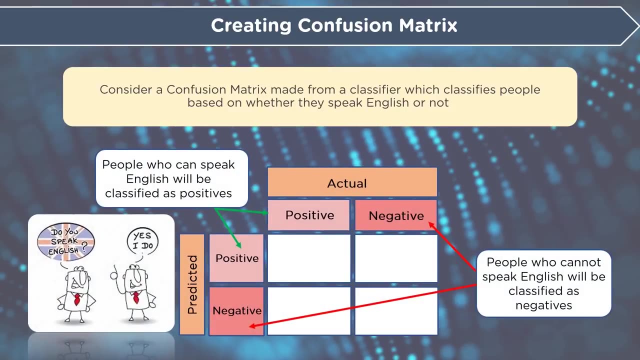 what this is based on its training. so we've already trained the model to guess whether it's spam or not spam or whatever it is you're working on, and then the actual values of our data set are along the columns. so this is the actual value that's supposed to be people who can speak english. 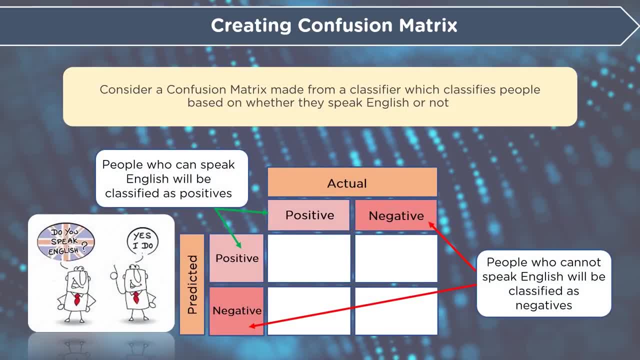 will be classified as positives. so, because they have a number zero or one, do you speak english? yes, no, and you could extend this that they might have. do you speak french? do you speak whatever languages you're going to use, but you're not going to use english, so you're going to use a whole lot of. 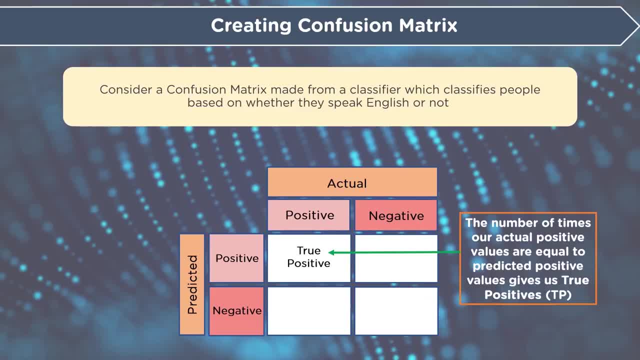 classifiers that you would look at. each one of these people who cannot speak english will be classified as negatives, so there'll be a zero. so you know zero ones. the number of times our actual positive values are equal to predicted positive values gives us true positive tp. the number of 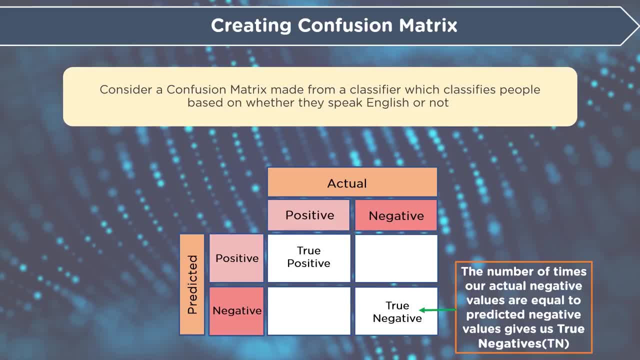 times our actual negative values are equal to predictive negative values gives us true negative tn. the number of times our model wrongly predicts negative values as positives is a false positive fp and you'll see when you're working with these a lot you know memorizing that is false positive. you can easily figure out what that is and pretty 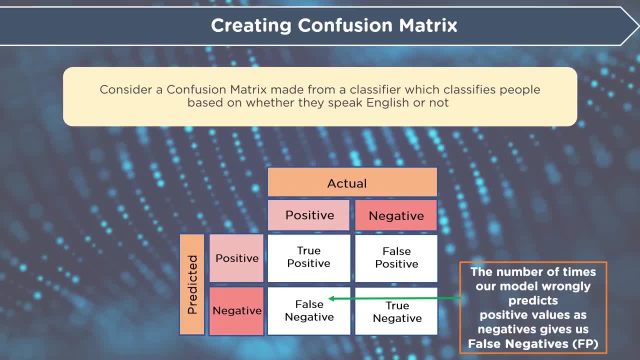 soon. you're just looking at the fp or the tp, depending on what you're working on and the numbers times. our model wrongly predicts positive values as negatives, gives us a false negative fp. now i'm going to do a quick step out here. let's say you're working in the medical and we're 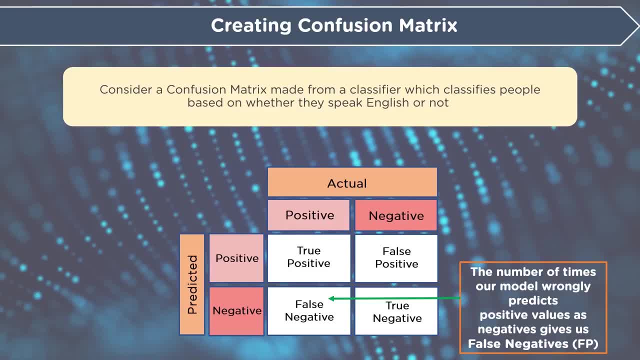 talking about cancer. do you really want a bunch of false negatives? you want zero under false negative. so when we look at this confusion matrix, if you have five percent false positives and five percent false negatives, it'd be much better to even have 20 false positives because they go in. 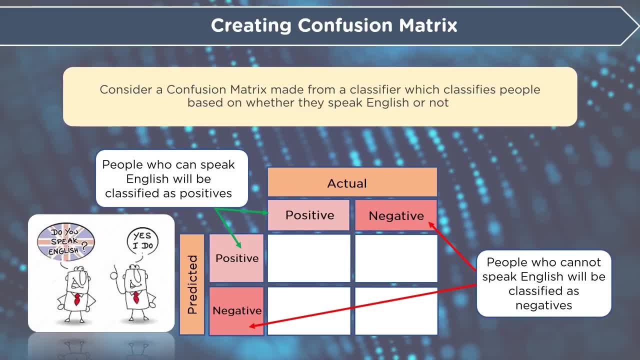 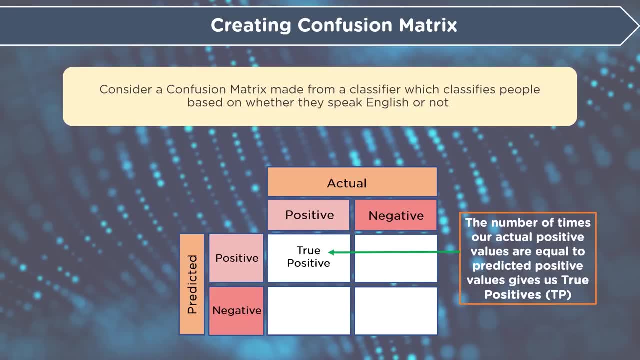 one of these People who cannot speak English will be classified as negatives, So there'll be a zero. So you know zero ones. The number of times our actual positive values are equal to predicted positive values gives us true positive TP. The number of times our actual negative values are equal to predictive. 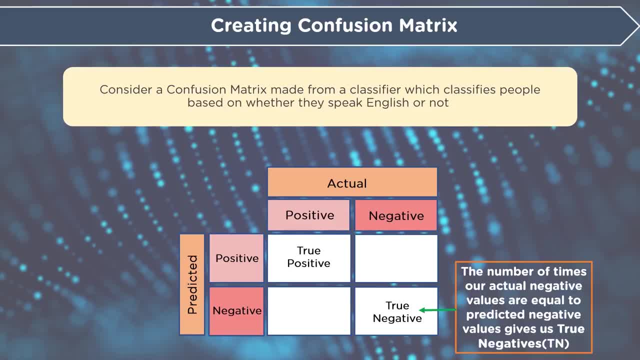 negative values gives us true negative TN. The number of times our model wrongly predicts negative values as positives gives us a false positive FP. And you'll see when you're working with these a lot, you know memorizing- that is false positive. you can easily figure out what. 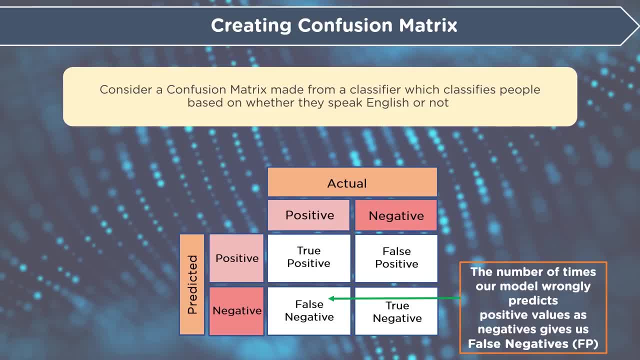 that is, and pretty soon. you're just looking at the FP or the TP, depending on what you're working on And the number of times our model wrongly predicts positive values as negatives gives us a false, negative FP. Now I'm going to do a quick step out here. Let's say you're working in the medical 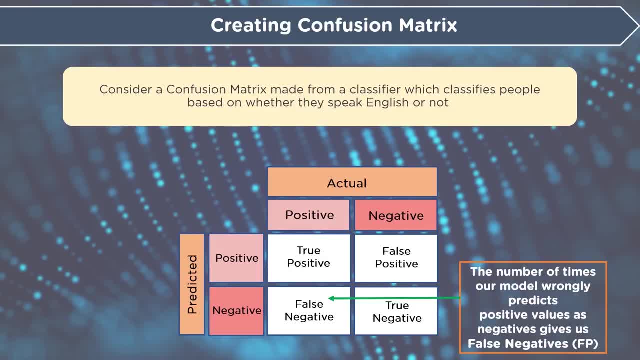 and we're talking about cancer. Do you really want a bunch of false negatives? You want zero under false negative. So when we look at this confusion matrix, if you have 5% false positives and 5% false negatives, it'd be much better to. 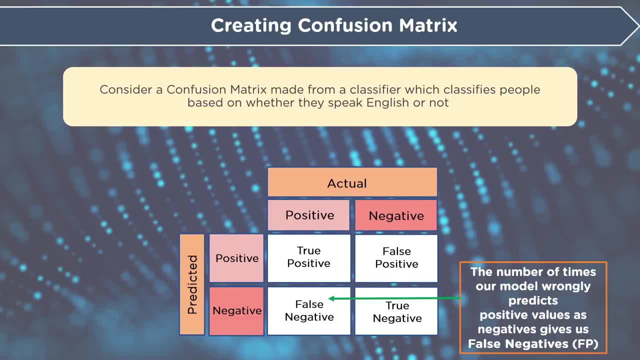 even have 20% false positives because they go in and test it, and zero false negatives. The same might be true if you're working on, say, a car driving. Is this a safe place for the car to go? Well, you really don't want any. 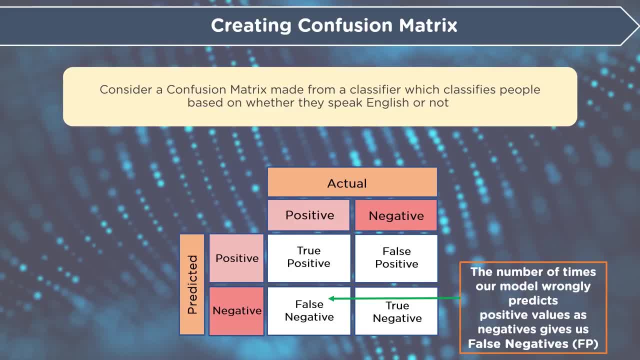 false positives. You know, yes, this is safe right over the cliff. So, again, when you're working on the project, or whatever it is you're working on, this chart suddenly has huge value. We were talking about spam email. How many important. 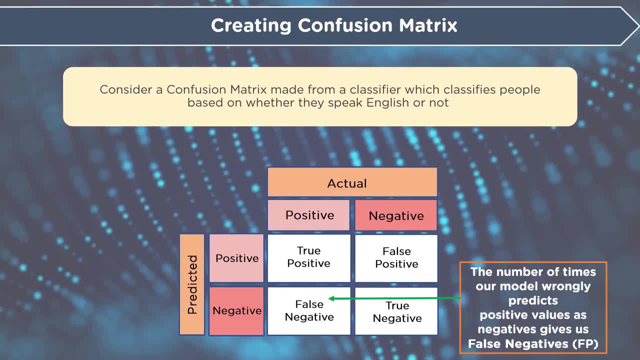 emails say from your banking overdraft charge coming in, that you want to be a true false negative. You don't want it to go in the spam folder. Likewise, you want to get as much of the spam out of there, but you don't want to. 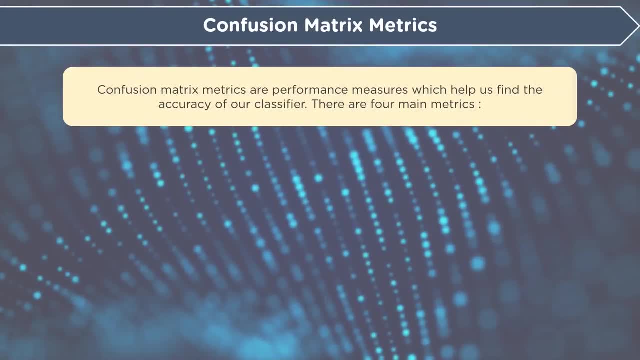 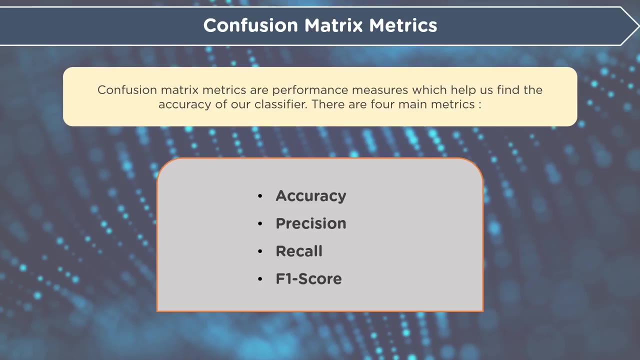 miss anything really important. Confusion matrix metrics are performance measures which help us find the accuracy of our classifier. There are four main metrics: accuracy, precision, recall and F1 score. The F1 score is the one I usually hear the most and accuracy is usually what you put on your chart when you're sending. 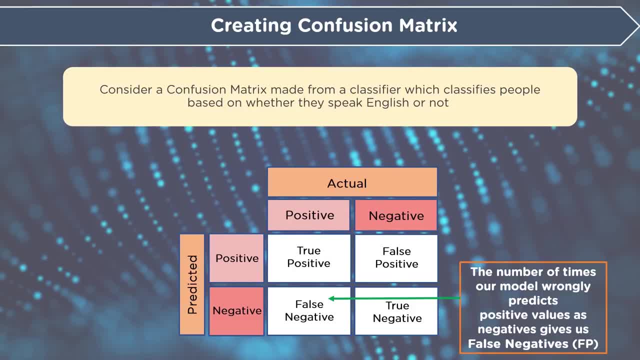 and test it in zero false negatives. the same might be true if you're working on, uh say, a car driving. this is a safe place for the car to go. well, you really don't want any false positives, you know, yes, this is safe right over the cliff. so again, when you're working on the project or whatever, 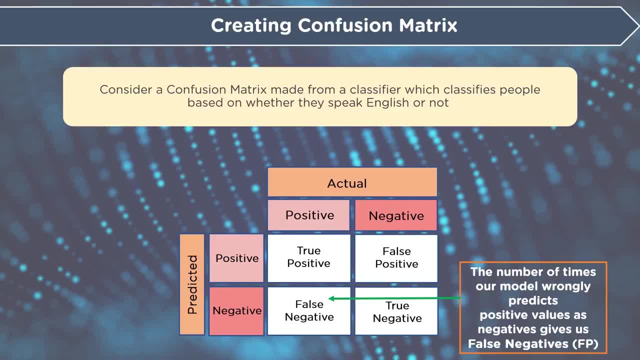 it is you're working on. this chart suddenly has huge value. we were talking about spam email. how many important emails, say from your banking overdraft charge coming in, that you want to be a a true, a false negative? you don't want it to go in the spam folder. likewise, you want to get the 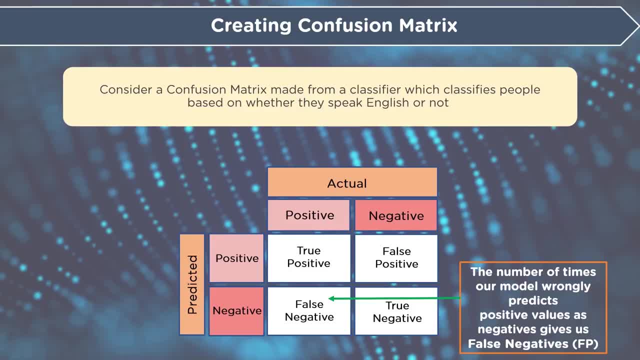 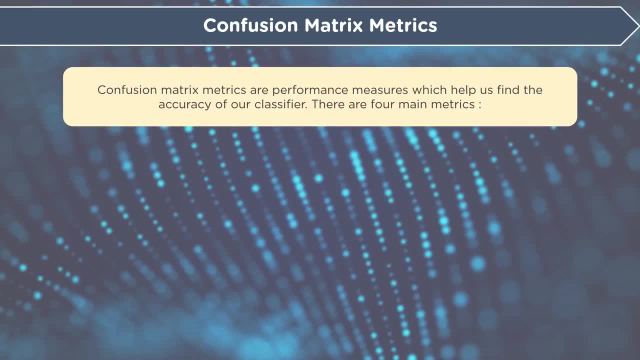 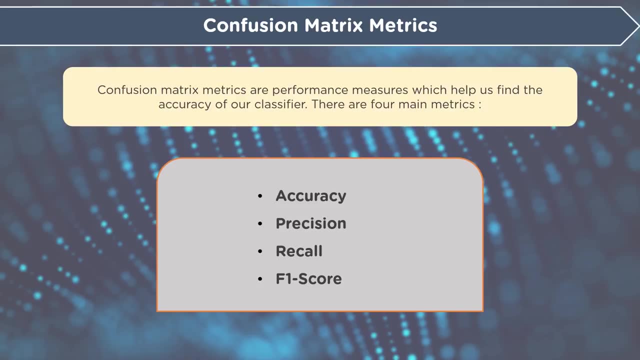 as much of the spam out of there, but you don't want to miss anything really important confusion. matrix metrics are performance measures which help us find the accuracy of our classifier. there are four main metrics: accuracy, precision, recall and f1 score. the f1 score is the one i 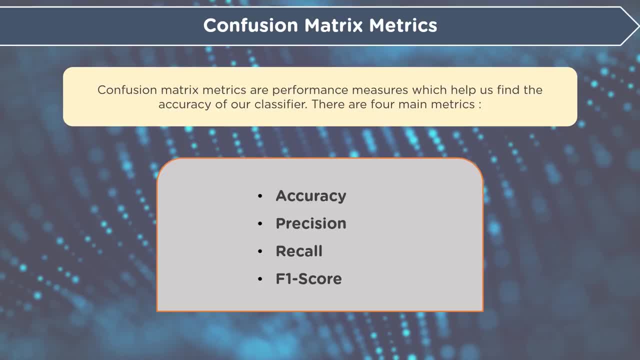 usually hear the most, and accuracy is usually what you put on your chart when you're sending in front of the shareholders. how accurate is it? people understand accuracy. um f1 score is a little bit more on the math side and so you have to be a little careful when. 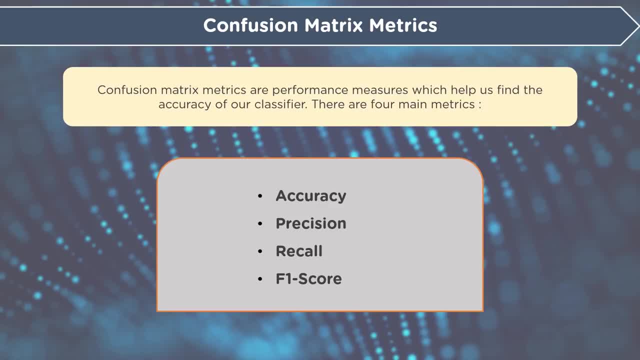 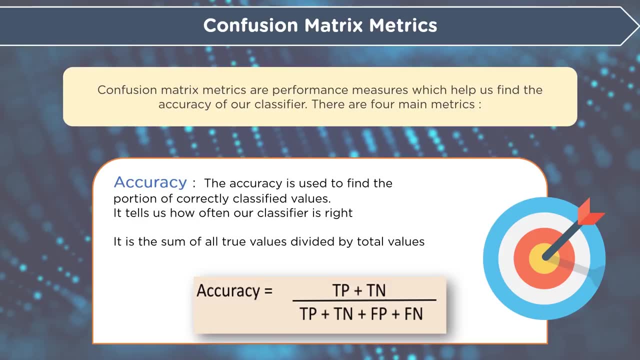 you're quoting f1 scores in the when you're sitting there with all the shareholders, because a lot of them will just glaze over, so confusion. matrix metrics are performance measures which help us find the accuracy of our classifier. there are four main metrics: accuracy: the accuracy is used to. 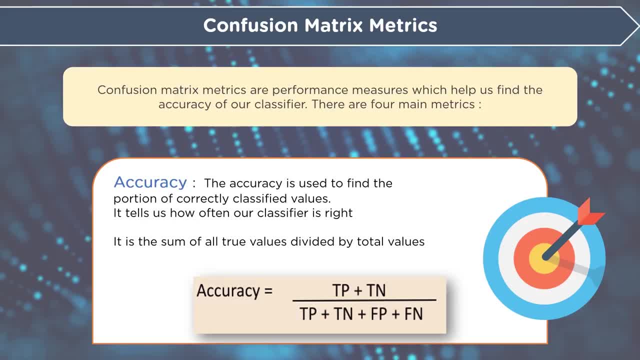 find the portion of the correctly classified values. it tells us how often our classifier is right. it is the sum of all true values, but it also tells us how much of a classifier we are classifying divided by the total values, and this makes sense. again, it's one of those. 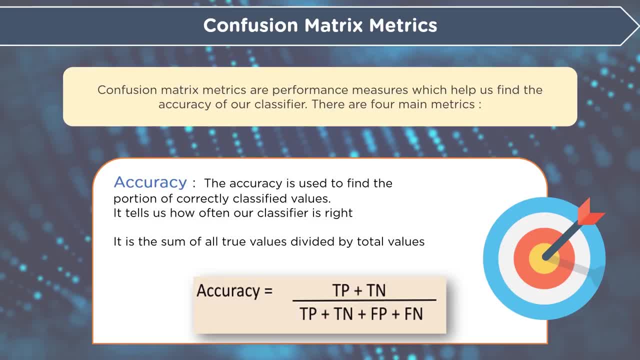 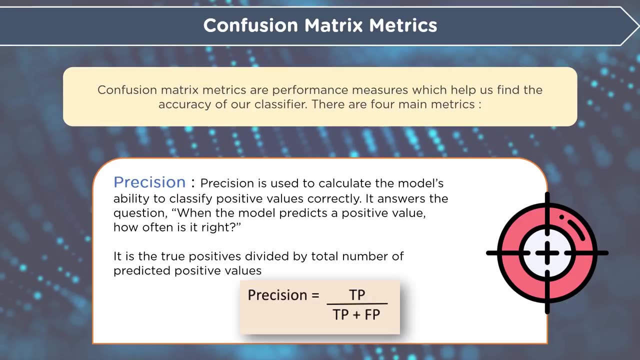 things I don't want to. you know what depends on what you're looking for. are you looking for not to miss any spam mails? are you looking to drive down the road and not run anybody over? precision is used to calculate the models ability to classify positive values correctly. it answers the question when the model 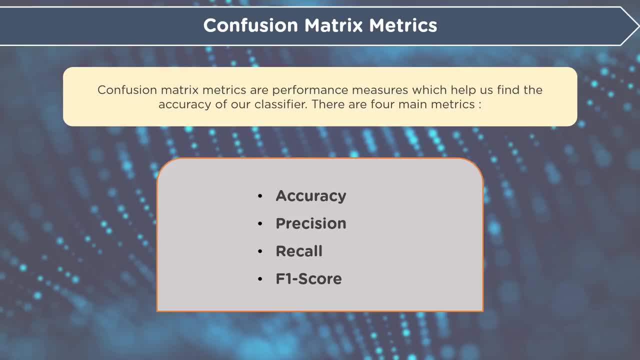 in front of the shareholders. How accurate is it? People understand accuracy. F1 score is a little bit more on the math side and so you have to be a little careful when you're quoting F1 scores when you're sitting there with all the shareholders, because a lot of them will just glaze over. So 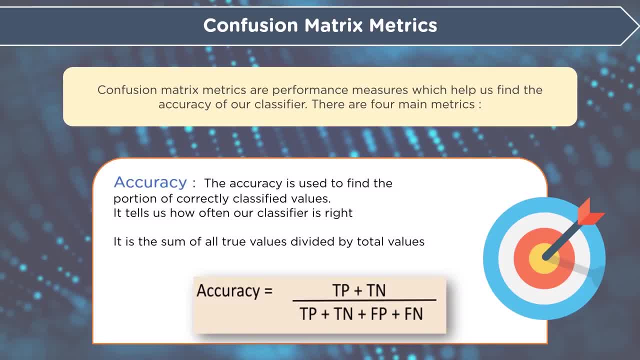 confusion. matrix metrics are performance measures which help us find the accuracy of our classifier. There are four main metrics: Accuracy: The accuracy is used to find the portion of the correctly classified values. It tells us how often our classifier is right. It is the sum of all true values divided by the total values, And this 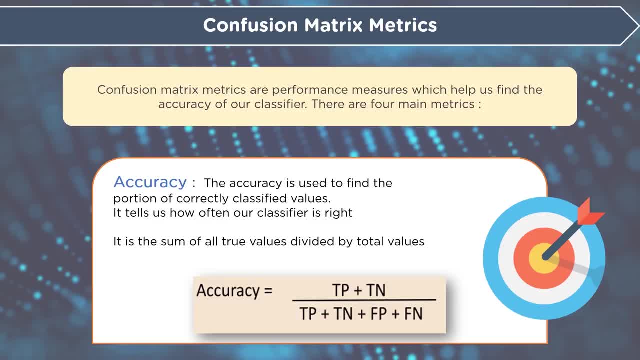 makes sense. Again, it's one of those things I don't want to. you know it depends on what you're looking for. Are you looking for not to miss any spam mails? Are you looking to drive down the road and not run anybody over? Precision. 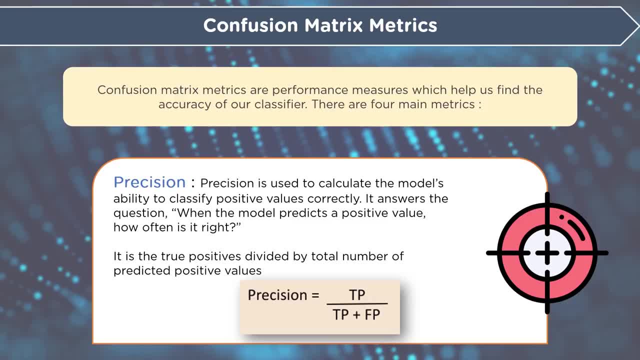 is used to calculate the model's ability to classify positive values correctly. It answers the question: when the model predicts a positive value, how often is it right? It is the true positive divided by the total number of predicted positive values. Again, this one depends on what project you're working on. 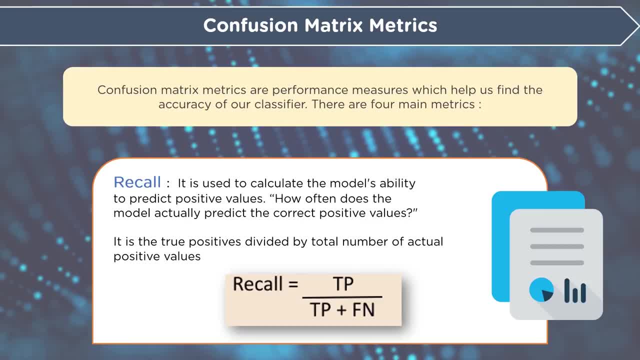 whether this is what you're going to be focusing on. So recall, it is used to calculate the model's ability to predict positive values. How often does the model actually predict the correct positive values? It is the true positive divided by the total number of actual positive values. 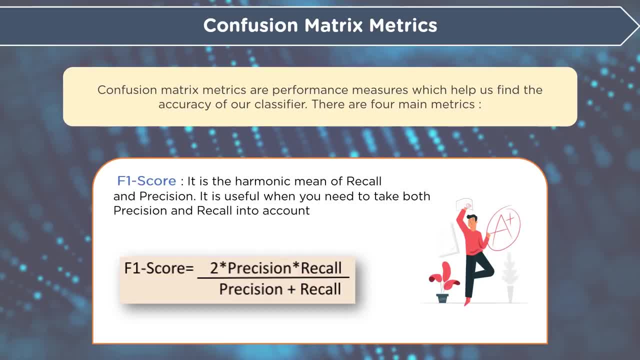 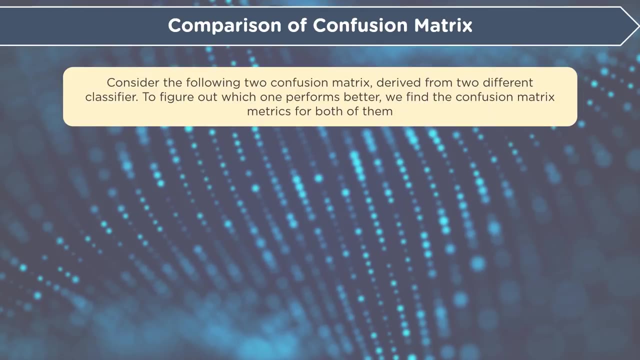 And then your F1 score. It is the harmonic mean of recall and precision. It is useful when you need to take both precision and recall into account. Consider the following two confusion matrix derived from two different classifier To figure out which one performs better. we can find the 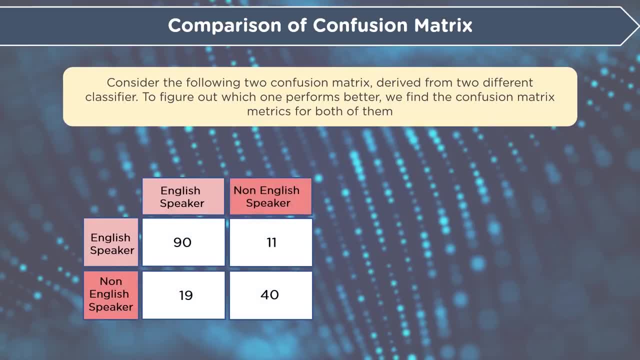 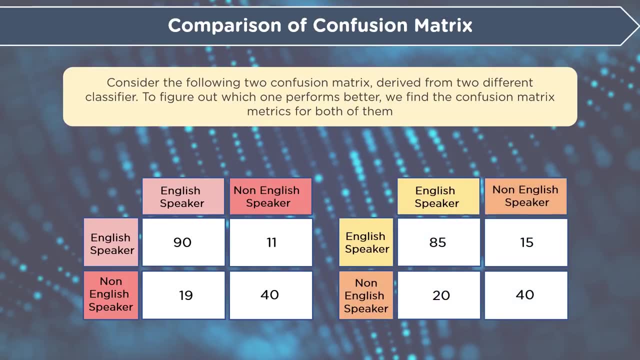 confusion matrix for both of them And you can see we're back to. does it classify whether they can speak English or are non-speaker? They speak something. they don't know- the English language- And so we put these two confusion matrices out here. We can go ahead and do the. 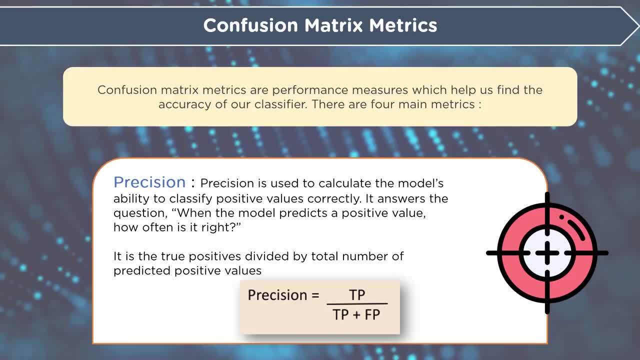 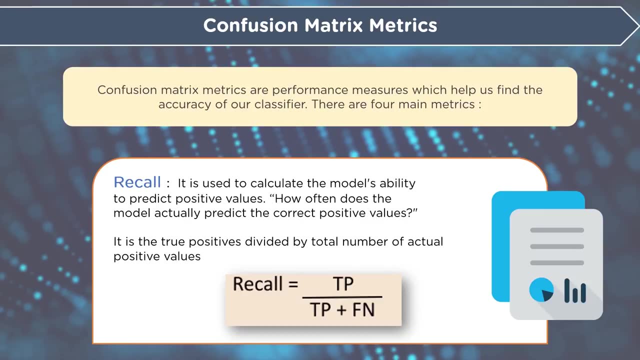 predicts a positive value. how often is it right? it is the true positive divided by the total number of predicted positive values. again, this one depends on what project you're working on, whether this is what you're going to be focusing on. so recall, it is used to calculate the model's ability to predict. 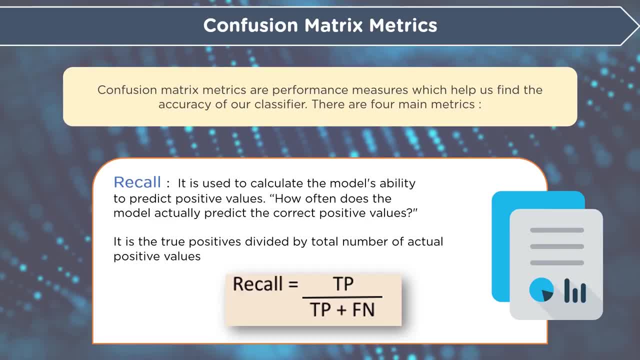 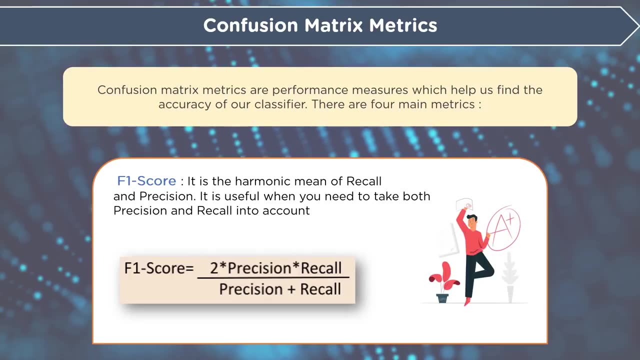 positive values. how often does the model actually predict the correct positive values? it is a true positive divided by the total number of attributes, actual positive values and then your f1 score. it is the harmonic mean of recall and precision. it is useful when you need to take both precision and recall into. 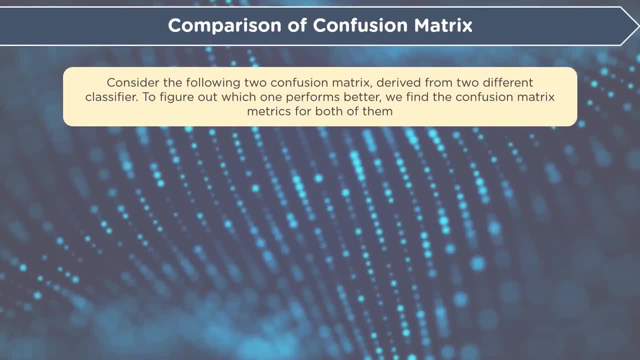 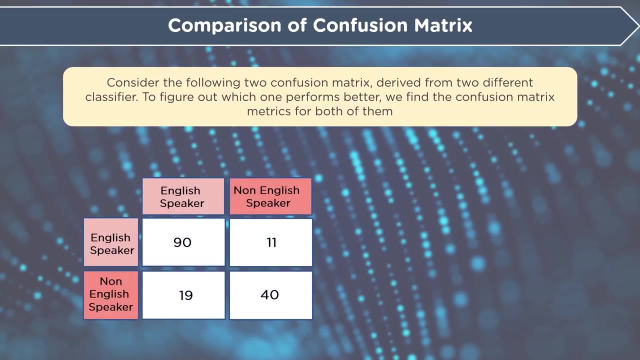 account. consider the following two confusion matrix derived from two different classifier to figure out which one performs better. we can find the confusion matrix for both of them and you can see we're back to. does it classify whether they can speak English or our nonspeak, or they speak something I don't? 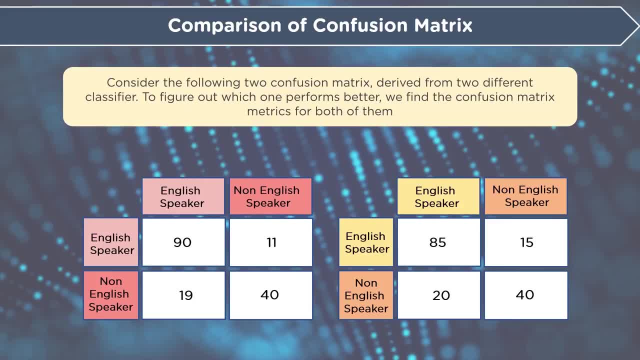 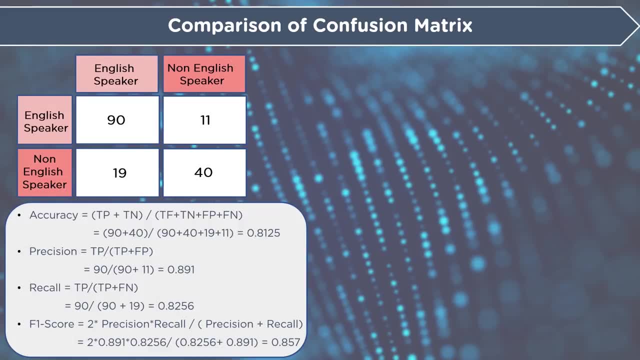 know the English language, and so we put these two confusion matrixes out here. we can go ahead and do the math behind that. we can look up the accuracy. that's a TPN plus tun over the TF plus t and plus f, p plus FN, and so we get an accuracy of. 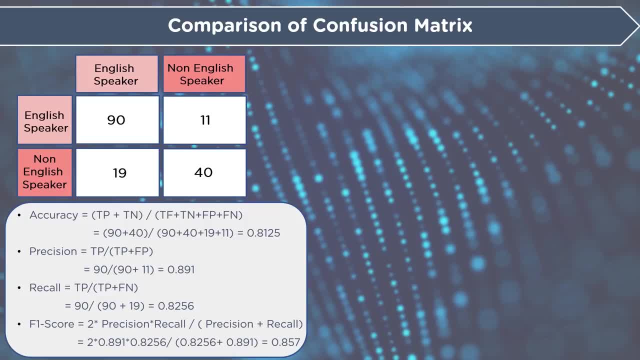 0. 햅 1, 2, 5 and we have a precision. if you do the precision, which is your TP truth positive over TP? Lタ-2 То Prop July beltEDA- plus FP, we get 0.891 and if we do the recall, we'll end up with the 0.825 that's your TP over TP plus. 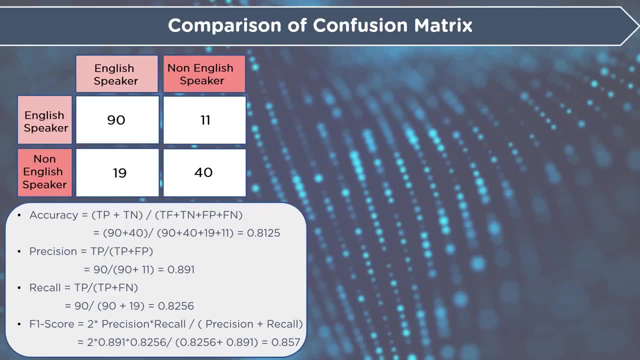 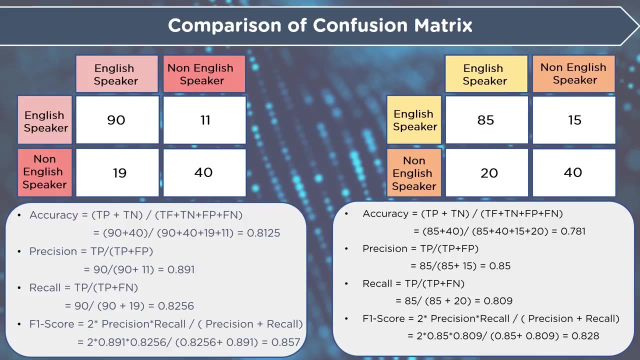 FN. and then of course, your F1 score, which is two times precision times, recall over precision plus recall, and we get the 0.857. and if we do that with another model- let's say we had two different models and we're trying to see which one we want to use for whatever reason- we might go ahead and 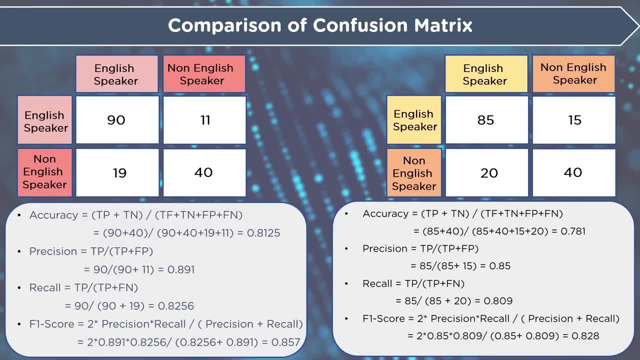 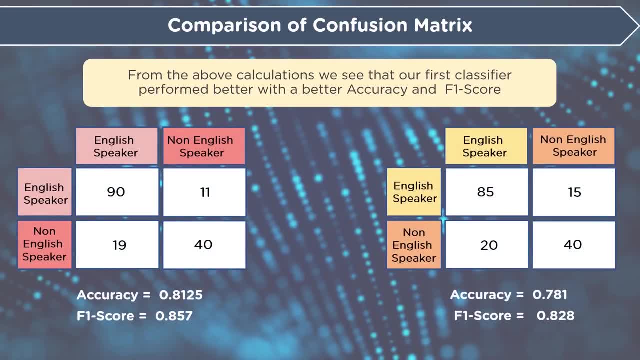 compute the same things. we have our accuracy, our precision and our recall and our F1 score and, as we're looking at this, we might look at the accuracy, because that's really what we're interested in is: how many people are we able to classify as being able to speak English? I really 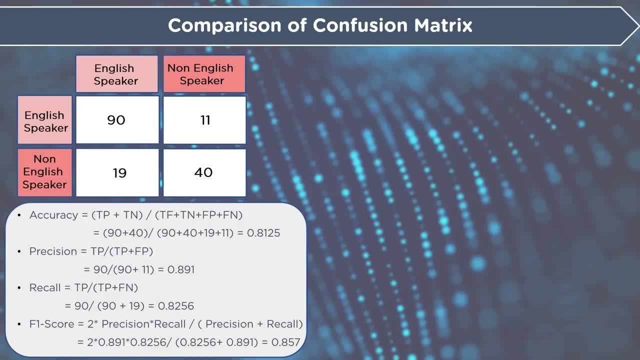 math behind that. We can look up the accuracy. That's a TPN plus TN over the TF plus TN plus FP plus FN, And so we get an accuracy of 0.8125.. And we have a precision. if you do the precision which is your TP truth positive over TP plus. 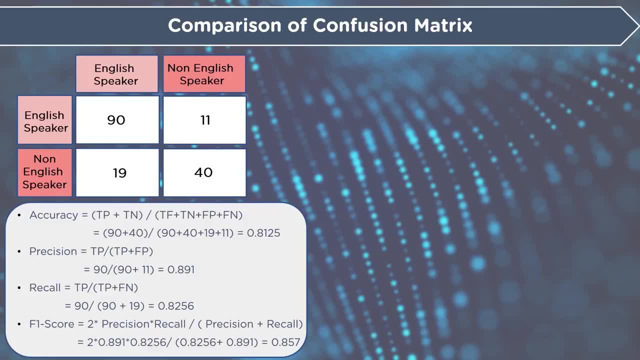 FP, get 0.891, and if we do the recall we'll end up with the 0.825, that's your TP over TP plus FN. and then of course, your F1 score, which is two times precision times recall over precision plus recall, and we get the 0.857. and if we do that with another model, let's say we had two different. 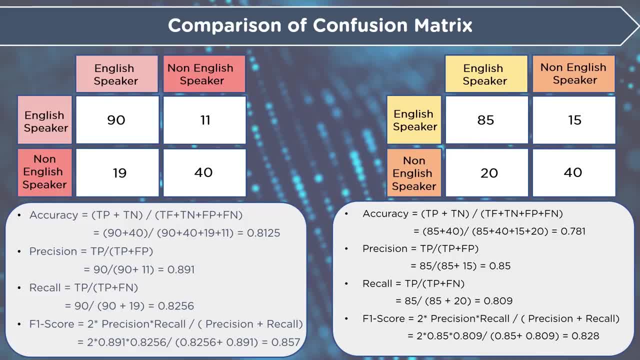 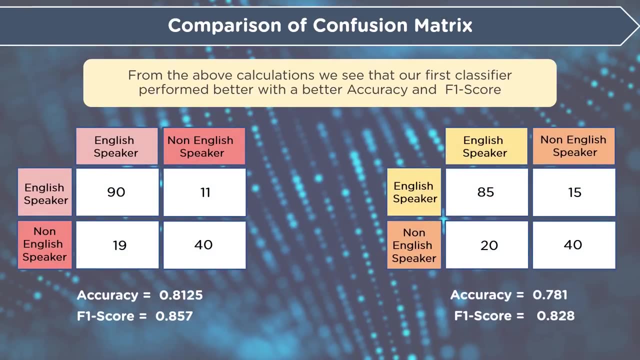 models and we're trying to see which one we want to use for whatever reason. we might go ahead and compute the same things. we have our accuracy, our precision and our recall and our F1 score and as we're looking at this, we might look at the accuracy, because that's really what we're. 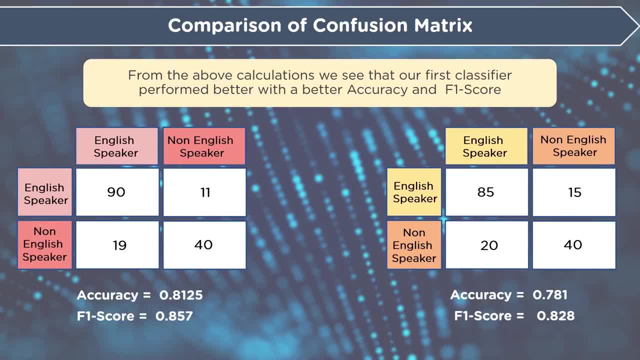 interested in is how many people are we able to classify as being able to speak English? I really don't want to know if I'm you know. I really don't want to know if they're non-speakers. I'd rather miss 10 people speaking English instead of 15, and so you can see from these charts we 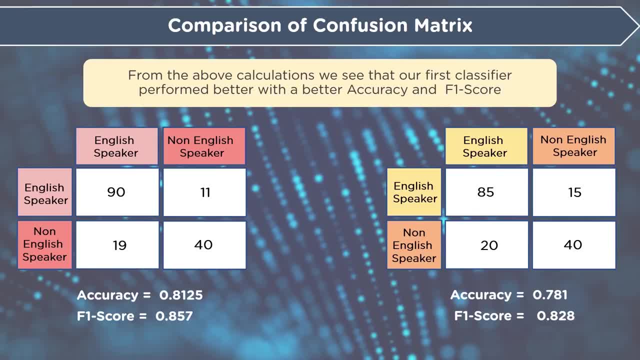 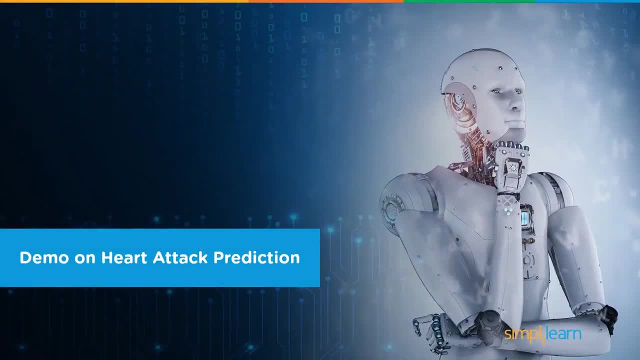 probably go with the first marginalized model, because it does a better job guessing who speaks English and has a higher accuracy, because in this case that is what we're looking for. so with that, we'll go ahead and pull up a demo so you can see what this looks like in. 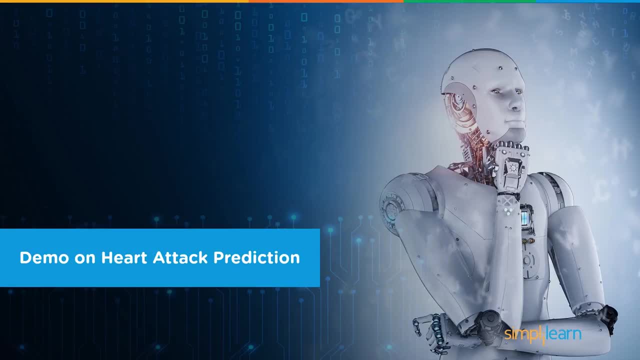 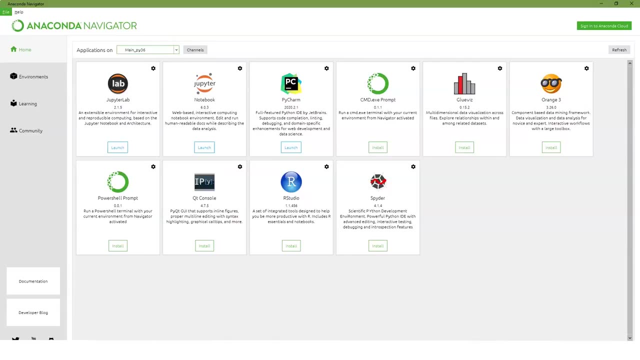 the Python setup in in the actual coding for this. we'll go into anaconda navigator. if you're not familiar with anaconda, it's a really good tool to use as far as doing display and demos and for quick development. as a data scientist, I just love the package. now, if you're going to do something heavier, 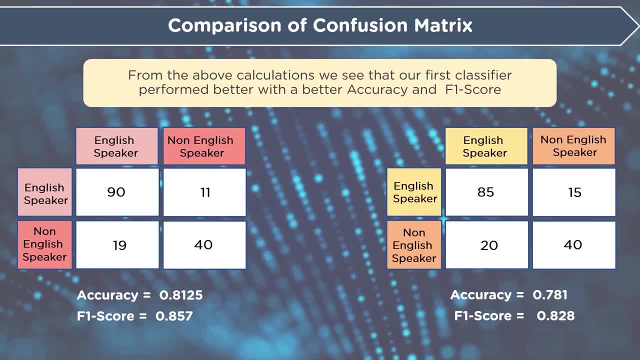 don't want to know if I'm. you know, I really don't want to know if they're non-speakers. I'd rather miss 10 people speaking English instead of 15, and so you can see from these charts, we probably go with the first model because it does a better job guessing who speaks English. 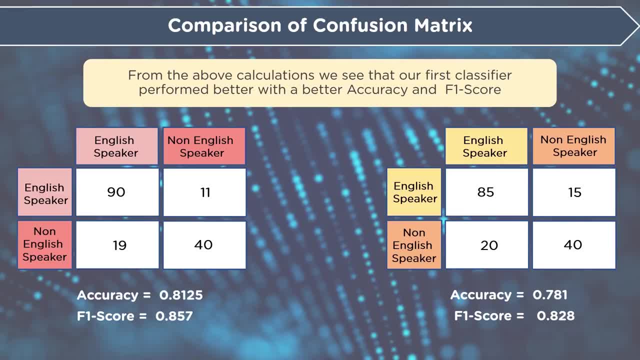 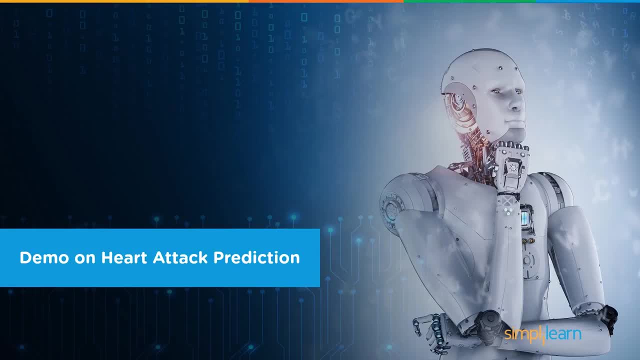 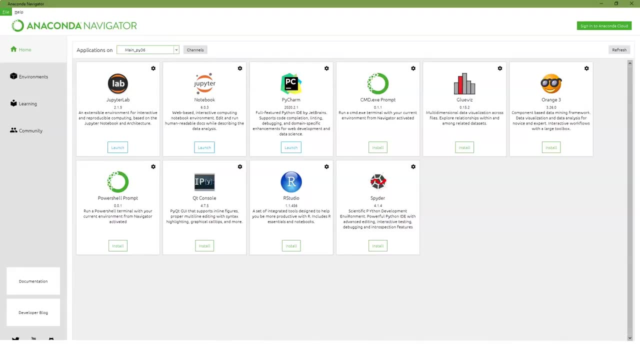 and has a higher accuracy, because in this case that is what we're looking for. so with that, we'll go ahead and pull up a demo so you can see what this looks like in the Python setup and in the actual coding. for this we'll go into Anaconda Navigator if you're not familiar with Anaconda. 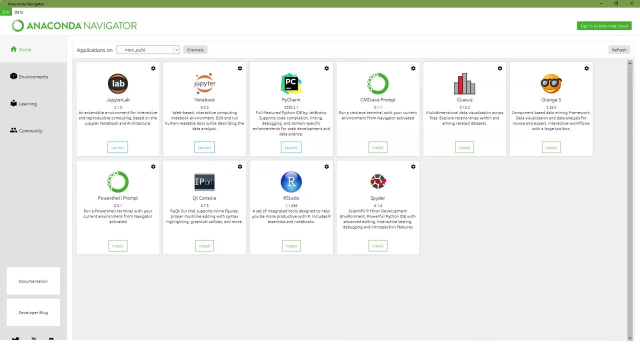 I'll show you how to do that in just a moment. but I'll show you how to do that in just a moment. it's a really good tool to use as far as doing display and demos and for quick development. as a data scientist, I just love the package. now, if you're going to do something heavier lifting, 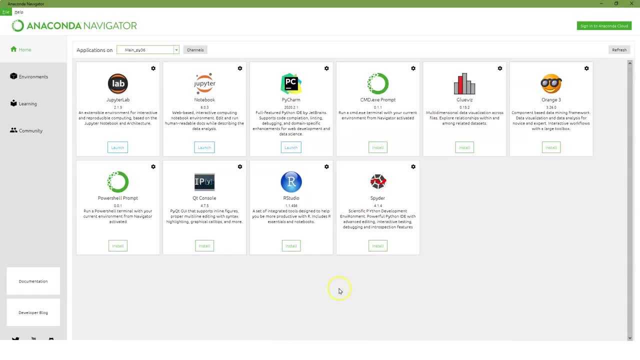 there's some limitations with Anaconda and with the setup, but in general you can do just about anything in here with your Python and for this we'll go with Jupyter Notebook. Jupyter Lab is the same as Jupyter Notebook. you'll see they now have integration with PyCharm if you work in PyCharm. 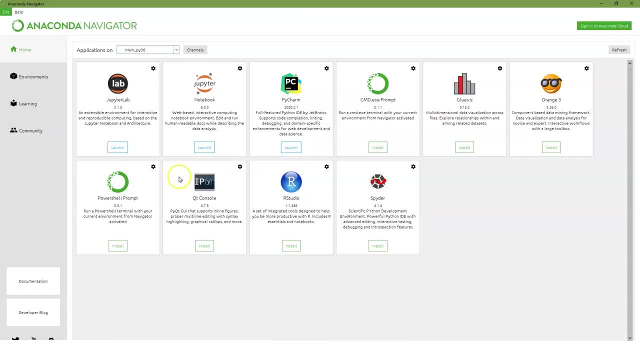 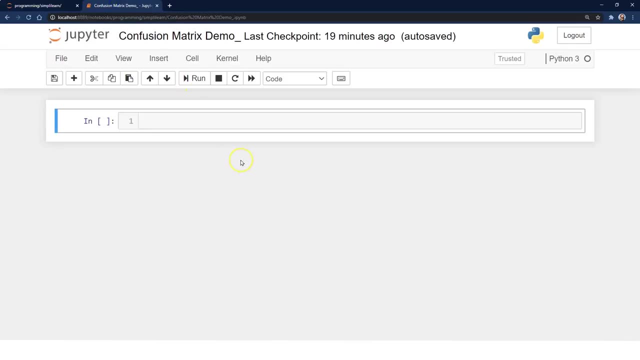 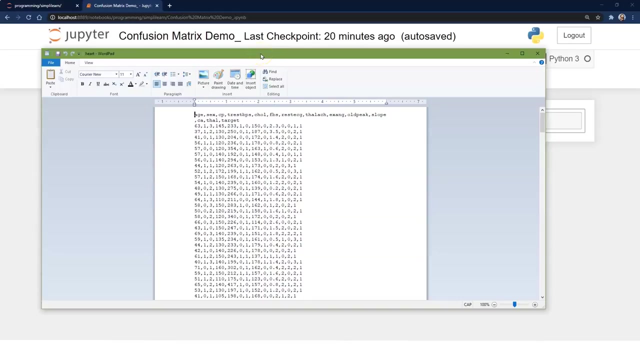 certainly there's a lot of other integrations that Anaconda has and we've opened up. simply learn files I work on and create a new file called confusion matrix demo, and the first thing we want to note is the data we're working with here. I've opened it up in a word pad or notepad or whatever. 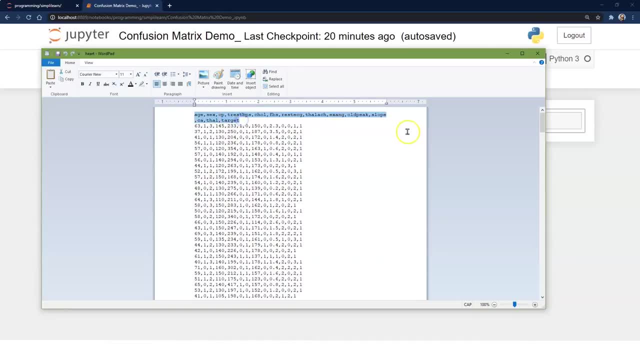 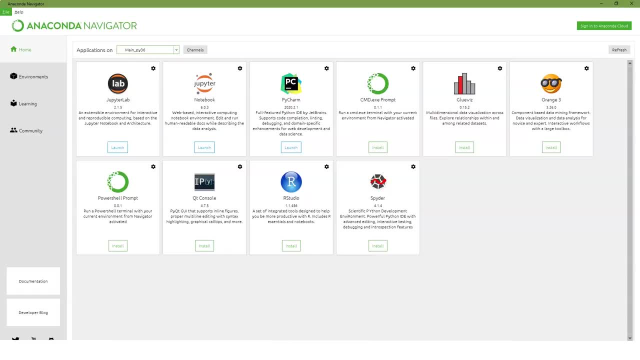 lifting. there's some limitations with anaconda and with the setup in general. you can do just about anything in here with your Python and for this we'll go with Jupyter notebook. Jupyter lab is the same as Jupyter notebook. you'll see they now have integration with PyCharm. if you work in PyCharm, certainly there's a lot. 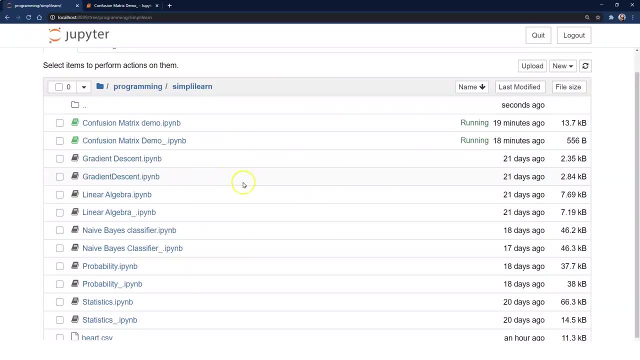 of other integrations that you can do with PyCharm if you work in PyCharm. there's also a lot of other integrations that anaconda has and we've opened up. simply learn files I work on and create a new file called confusion matrix demo. 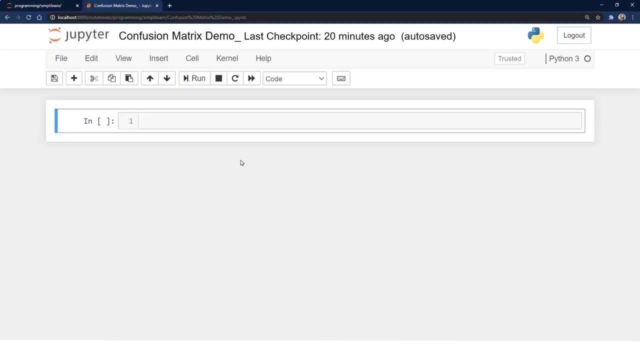 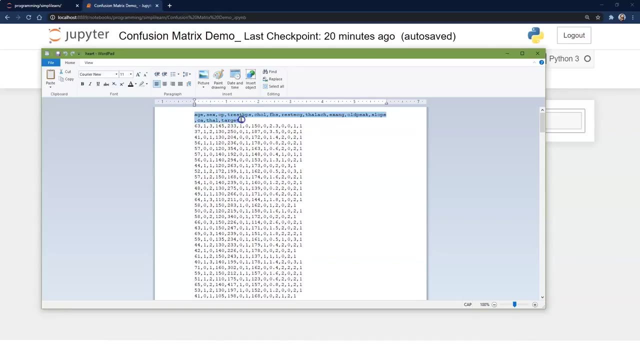 and the first thing we want to note is the data we're working with here. I've opened it up in a word pad or notepad or whatever. you can see it's got a row of headers comma separated, and then all the data going down below, and then I saved. 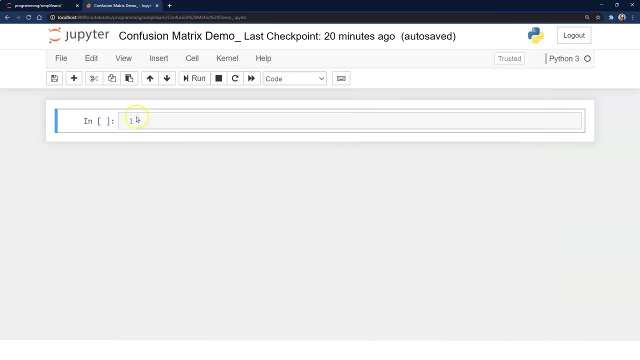 this in the same file, so I don't have to remember what path I'm working on working on. Of course, if you have your data separated and you're working with a lot of data, you probably want to put it into a different folder or file, depending on what you're doing. 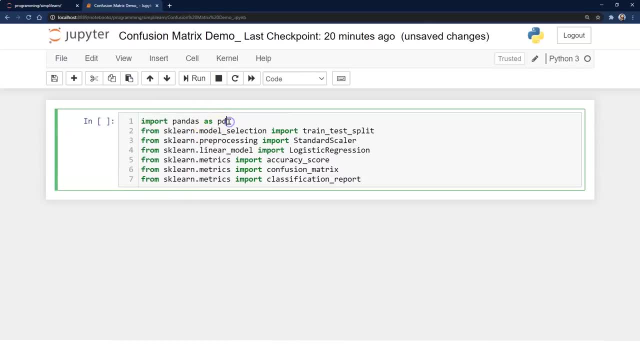 And the first thing we're going to do is go ahead and import our tools. We're going to use the pandas. That's our data frame. If you haven't had a chance to work with the data frame, please review panda's data frame and go into Simply Learn. You can pull up the panda's data frame tutorial on. 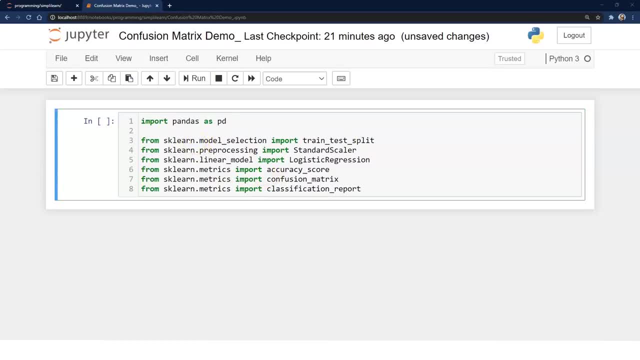 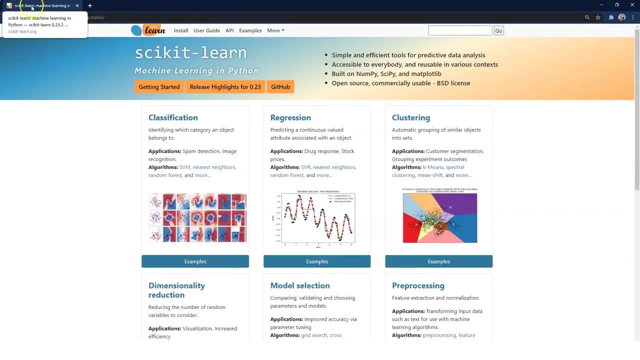 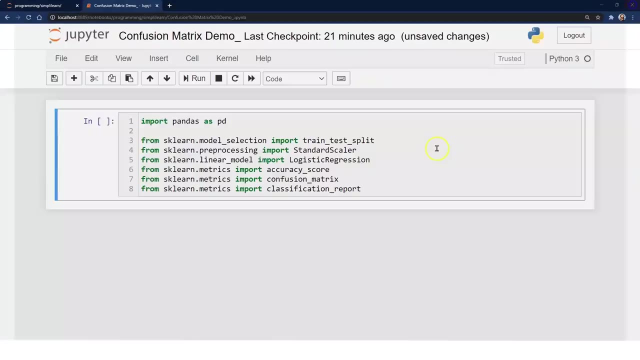 there, And then we're going to use the scikit framework, which is all denoted as sklearn, And I can just pull this in. You can see, here's the scikit-learnorg with the stable version that you can import into your Python, And from here we're going to use the train test split. 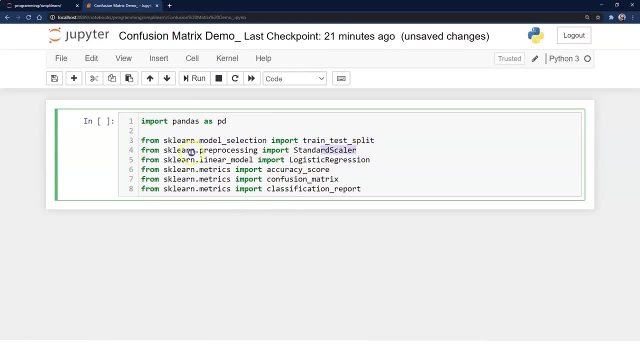 for splitting our data. We're going to do some pre-processing, We're going to use the logistic regression model. That's our actual machine learning model we're using, And then what this particular setup is about is we're going to do the accuracy score, the confusion matrix and the classifier. 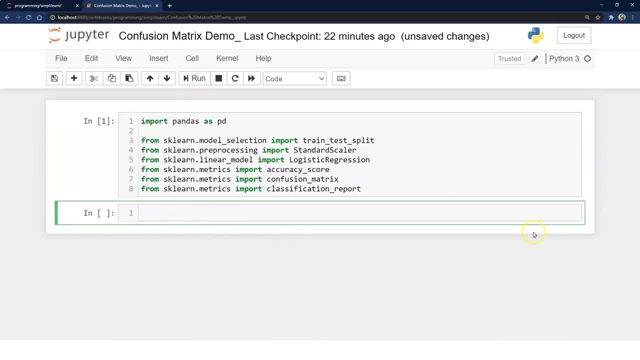 report. So let me go ahead and run that and bring all that information in And, just like we opened the file, we need to go ahead and load our data in here. So we're going to go ahead and do our pandas, read CSV And then, just because we're in Jupyter, 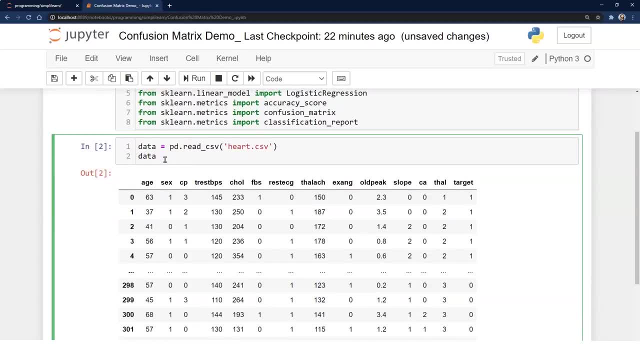 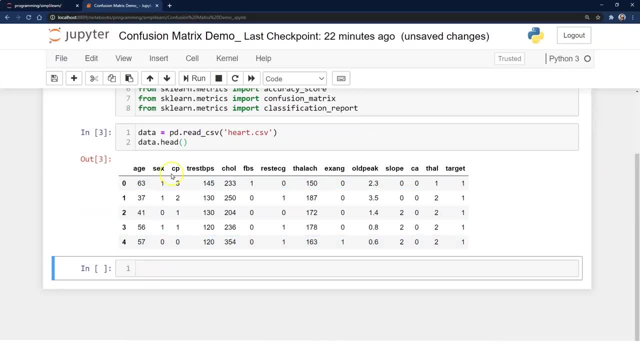 Notebook we can just put data to read CSV. So let me just read the data in here. A lot of times we'll actually let me just do this. I prefer to do just the head of the data, the top part, And you can see we have age six. I'm not sure what CP stands. 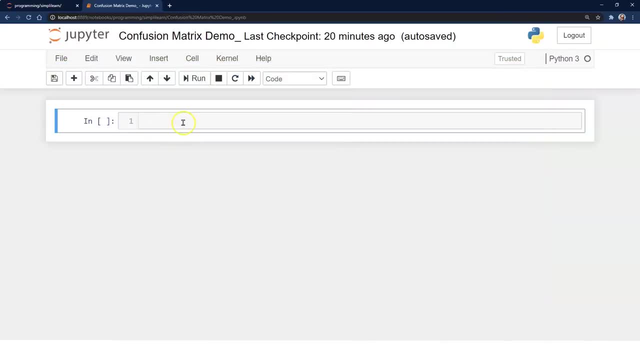 same file, so I don't have to remember what path I'm working on. of course, if you have your data separated and you're working with a lot of data, you probably want to put it into a different folder or file, depending on what you're doing, and the first thing we're going to do is go ahead and 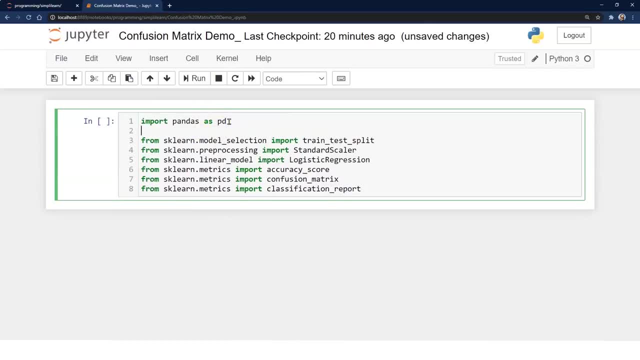 import our tools. we're going to use the pandas. that's our data frame. if you haven't had a chance to work with the data frame, please review pandas data frame and go into simply learn. you can pull up the pandas data frame tutorial on there and then we're going to use the. 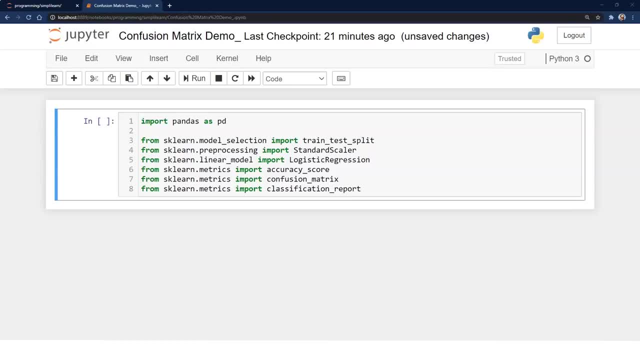 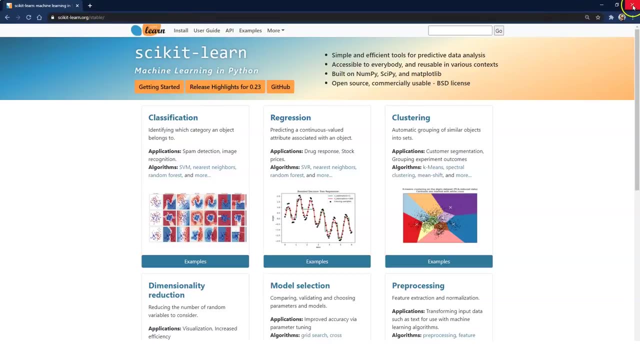 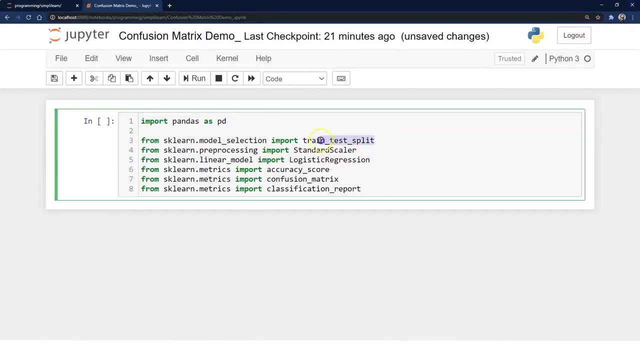 scikit framework, which is all denoted as sklearn, and I can just pull this in. you can see, here's the scikit-learnorg with the stable version that you can import into your Python and from here we're going to use the train test split for splitting our data. we're going to do some pre-processing. 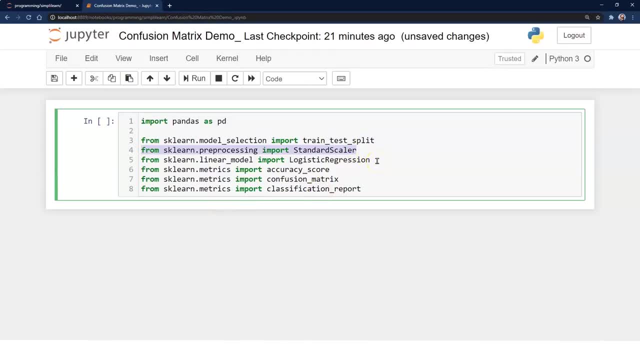 we're going to do use the logistic regression model. that's our actual machine learning model we're using, and then, with this core this particular setup is about, is we're going to do the accuracy score, the confusion matrix and the classifier report. so let me go ahead and run that and bring all that. 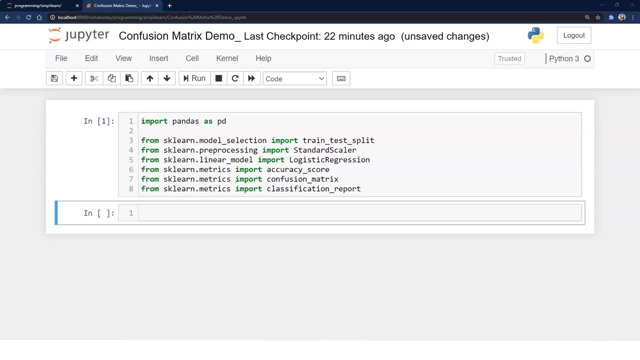 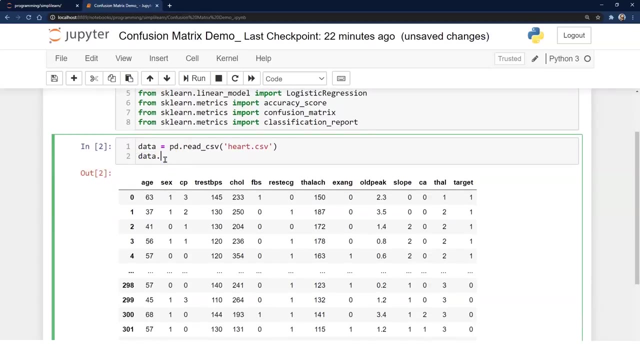 information in and just like we open the file, we need to go ahead and load our data in here. so we're going to go ahead and do our pandas, read csv, and then, just because we're in Jupyter notebook, we can just put data to read the data in here. a lot of times we'll actually let me just do this. 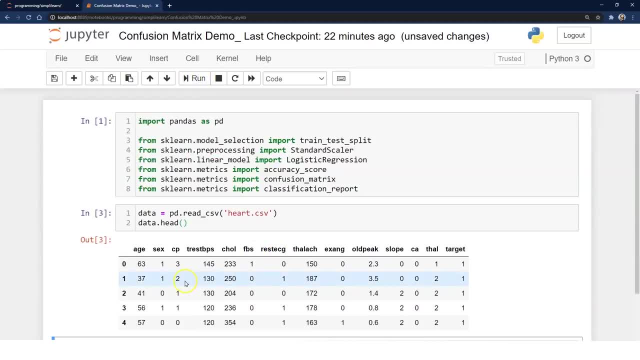 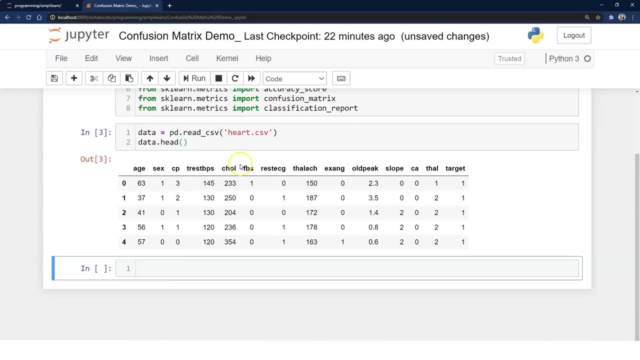 I prefer to do this- just the head of the date or the top part, and you can see we have age sex. I'm not sure what cp stands for, test bps, cholesterol. so a lot of different measurements. if you were in this domain, you want to know what all these different measurements mean. I don't want to focus on that too much because 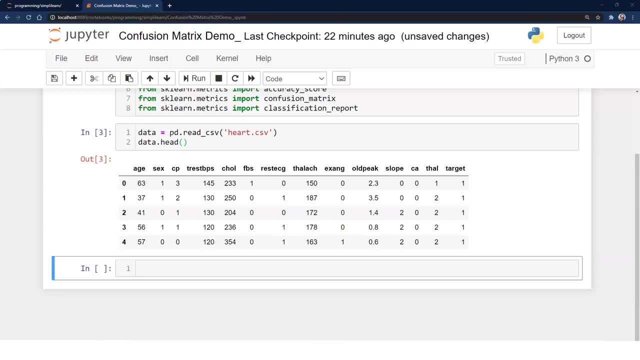 when we're talking about data science. a lot of times you have no idea what the data means. if you've ever looked up the breast cancer measurement, it's just a bunch of measurements and numbers. unless you're a doctor, you're going to have no idea what those measurements mean. but if it's your specialty in your domain, you better know them. 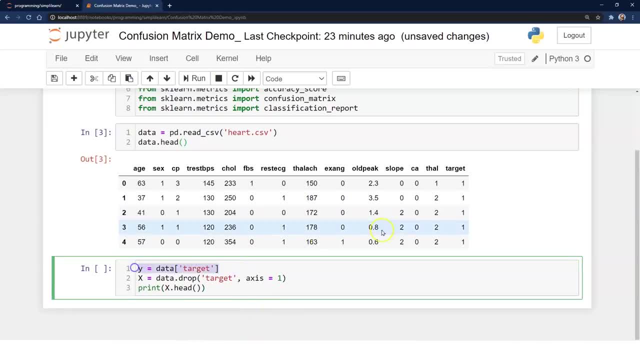 so we're going to go ahead and create y and it's going to. we're going to set it equal to the target. so here's our target value here, and it's either 1 or 0. so we have a classifier. if you're dealing with one- zero, true, false- what do you have? you have a classifier and then our x is: 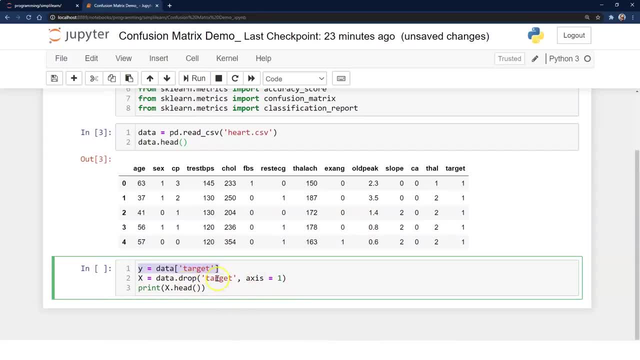 going to be everything except for the target. so we're going to go ahead and drop the target. axes equals 1.. remember that's columns versus the index or rows. axes equals 0 would would give you an error, but you would drop like row 2.. and then we'll go ahead. just print that. 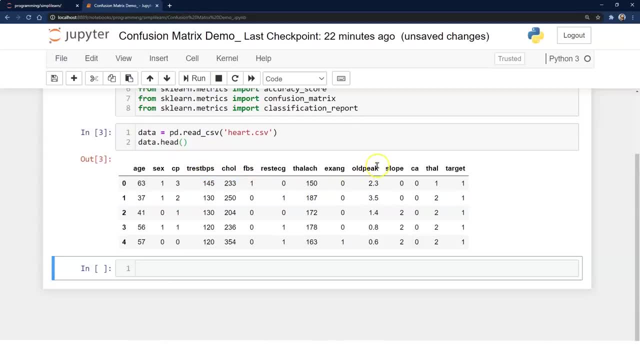 for test BPS cholesterol. So a lot of different measurements. If you were in this domain, you'd want to know what all these different measurements mean. I don't want to focus on that too much because when we're talking about data science, a lot of times you have no idea what the data science. 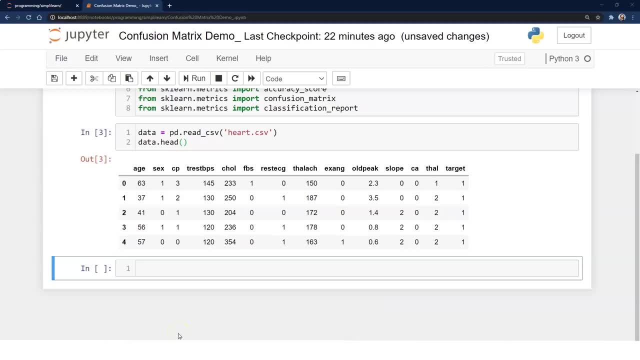 means If you've ever looked up the breast cancer measurement, it's just a bunch of measurements and numbers. Unless you're a doctor, you're going to have no idea what those measurements mean. But if it's your specialty in your domain, you better know them. So we're going to go ahead and create. 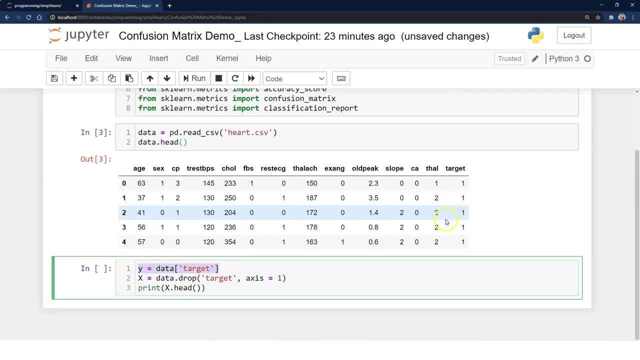 Y, and we're going to set it equal to the target. So here's our target value here, And it's either one or zero. So we have a classifier. If you're dealing with one, zero, true, false, what do you? 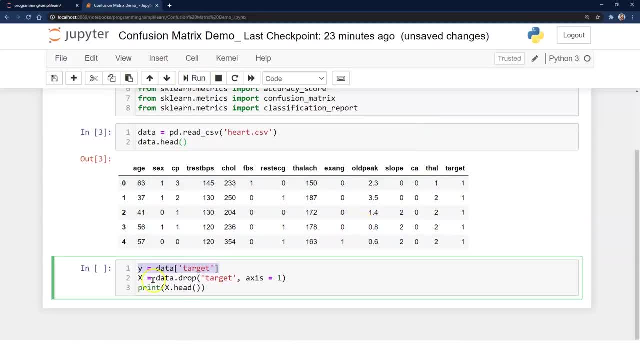 have. You have a classifier And then our X is going to be everything except for the target. So we're going to go ahead and drop the target. Axis equals one- Remember that's columns- versus the index or rows. Axis equals zero would give you an error, but you would drop like row two, And then 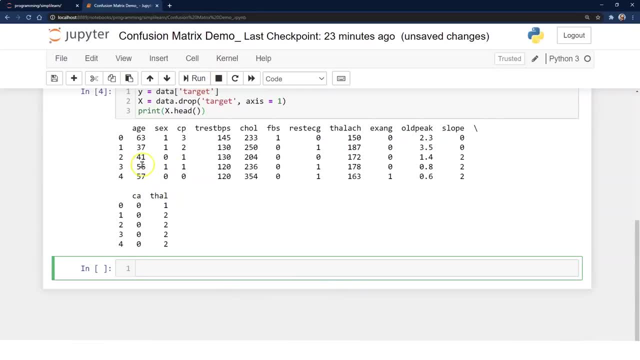 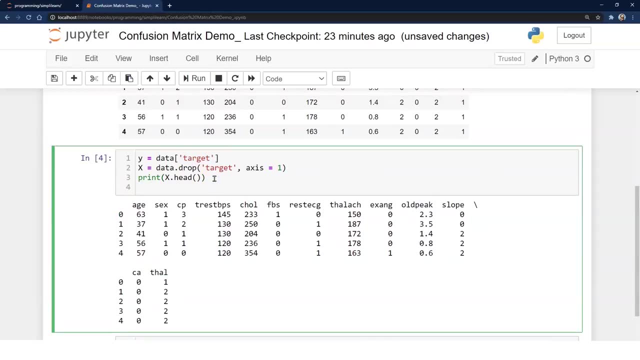 we'll go ahead and just print that out so you can see what we're looking at. And here we have Y data, X data And you can see from the X data we have the X head And we can go ahead and just do print the Y. 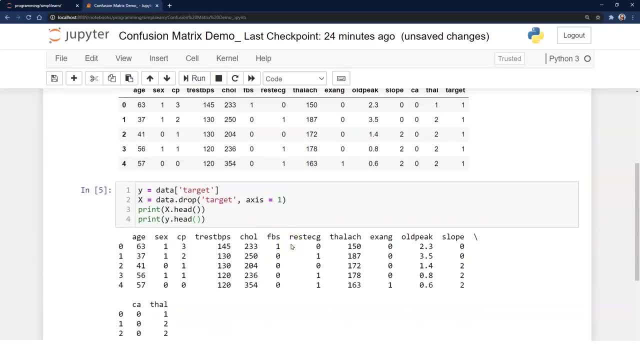 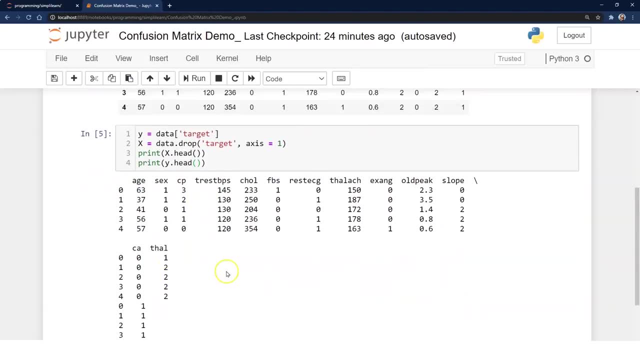 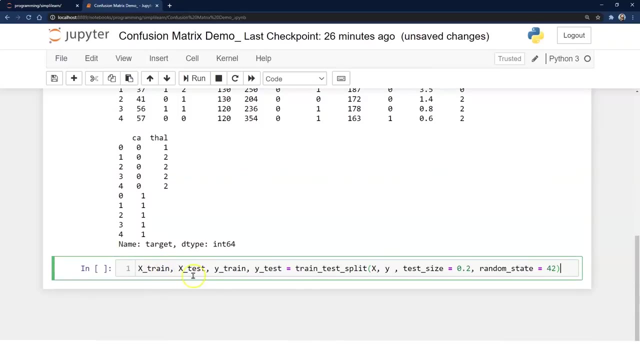 head data and run that. So this is all loading the data that we've done so far. If there's a confusion in there, go back and rewind the tape and review it, And then we need to go ahead and split our data into our X train, X test, Y train, Y test. 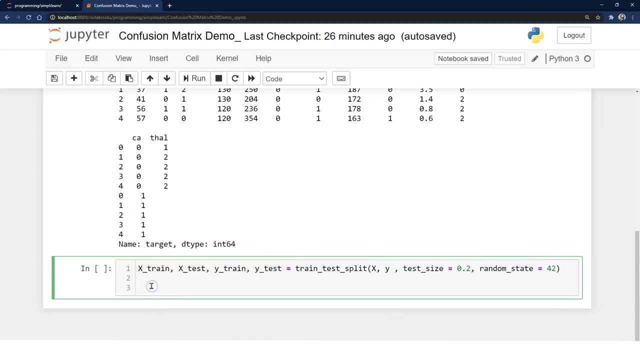 And then keep that in mind in mind. you always want to split the data before we do the scalar, and the reason is is that you want the scalar on the training data to be set on the training data data or fit to it, but not on the test data. think of this as being 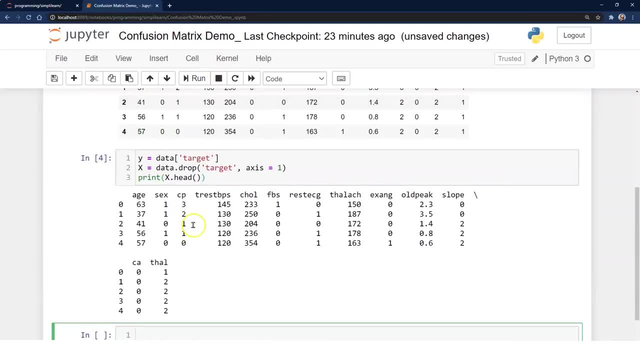 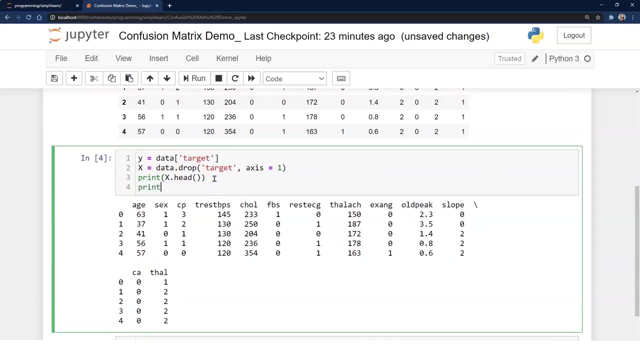 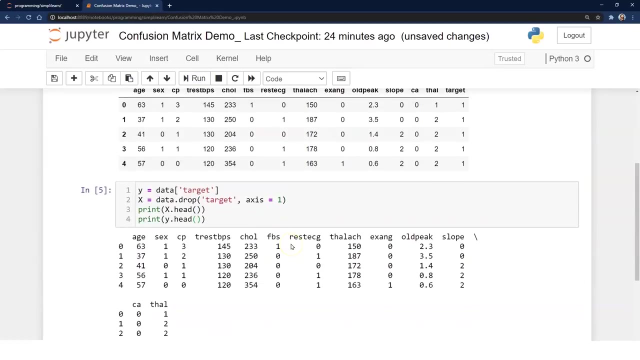 out so you can see what we're looking at. and, uh, here we have y data, x data and you can see from the x data we have the x head and we can go ahead and just do print x dot. we're going to bring down the Y head data and run that. So this is all loading the data that we've done so far. If 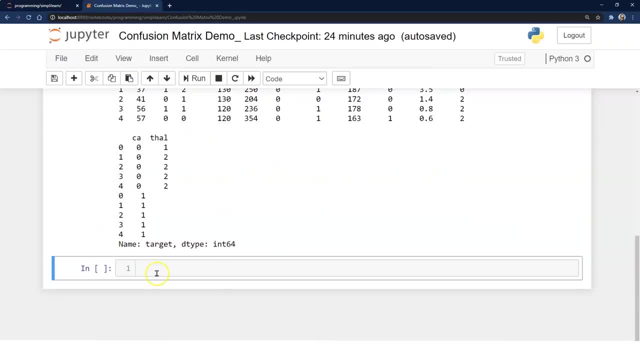 there's a confusion in there, go back and rewind the tape and review it And then we need to go ahead and split our data into our X train, X test, Y train, Y test And then, keep in mind, you always want to split the data before we do the scalar And the reason is that you want the scalar on the 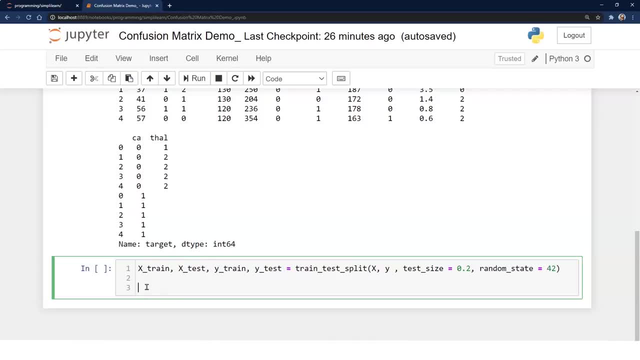 training data to be set on the training data or fit to it, but not on the test data. Think of this as being out in the field. It could actually alter your results. So it's always important to make sure whatever you do to the training data or whatever fit you're doing is always done on the 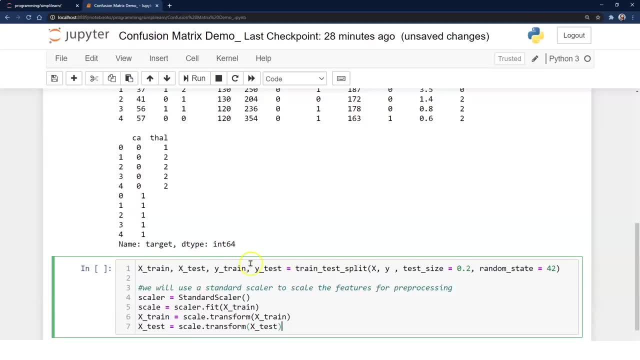 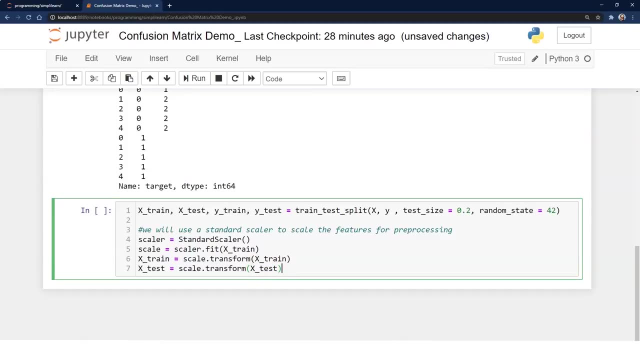 training, not on the test. And then we want to go ahead and scale the data. Now we are working with linear regression model. I'll mention this here in a minute when we get to the actual model. So sometimes you don't need to. 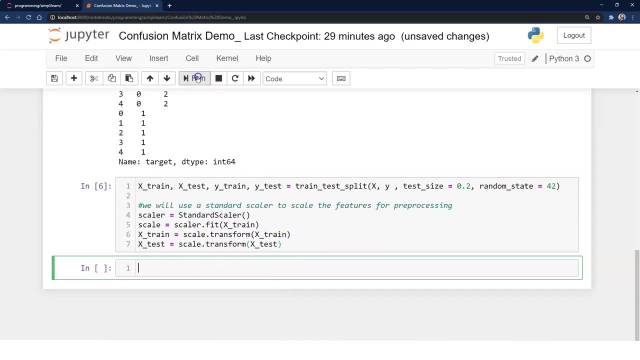 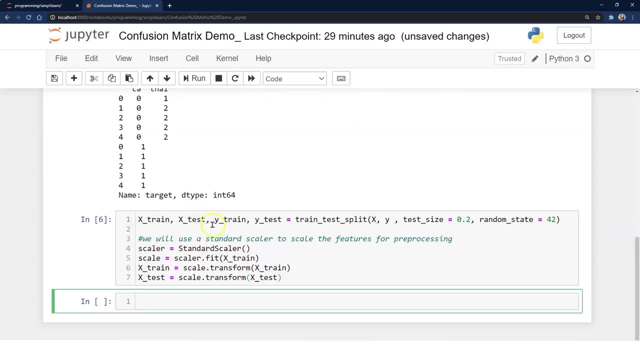 scale it. when you're working with linear regression models, It's not going to change your result, as much as, say, a neural network where it has a huge impact. But we're going to go ahead and take- here's our X train, X test, Y train, Y test. We create our scalar, We go ahead and scale. 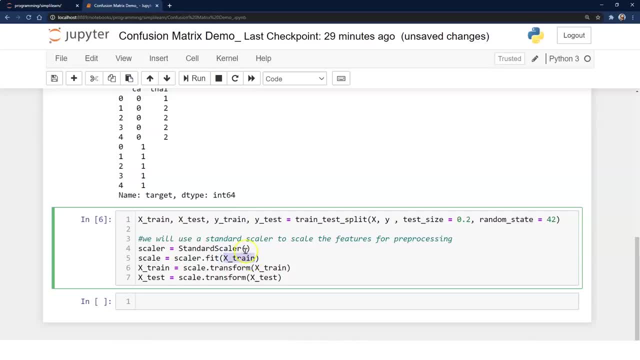 And then we want to go ahead and scale the data. Now we're going to go ahead and scale the data. The scale is going to fit the X train. And then we're going to go ahead and take our X train and transform it. And then we also need to take our X test and transform it based on the scale on here. 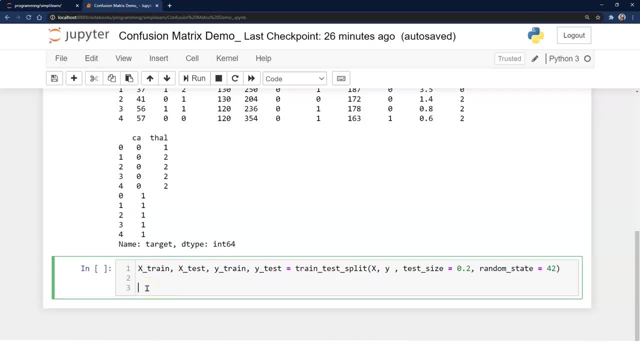 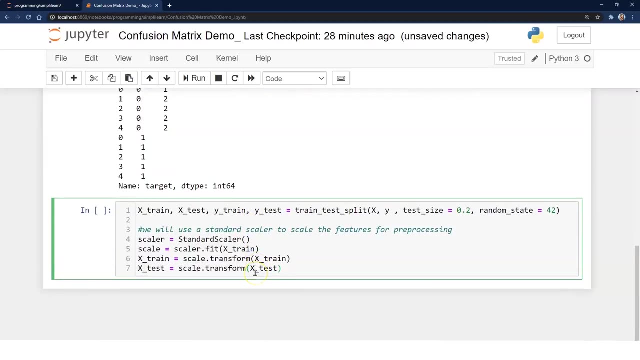 out in the field. you're not, it could actually alter your results. so it's always important to do make sure whatever you do to the training data, or whatever fit you're doing, is always done on the training, not on the test. and then we want to go ahead and scale the data. now we are working with linear. 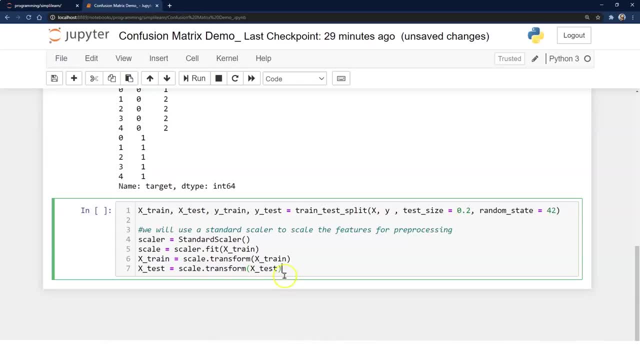 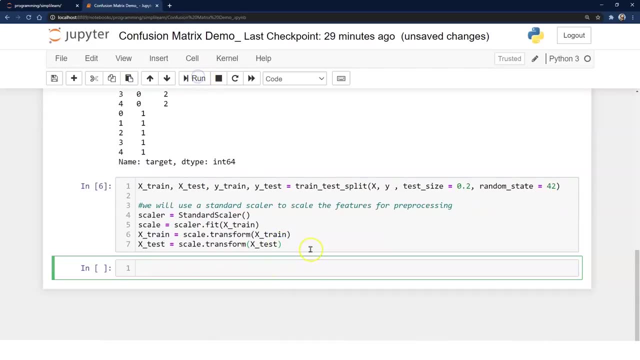 regression model. I'll mention this here in a minute when we get to the actual model. so some, but sometimes you don't need to scale it when you're working with linear regression models. it's not going to change your result as much as, say, a neural network where it has a huge impact. but we're going to go ahead and 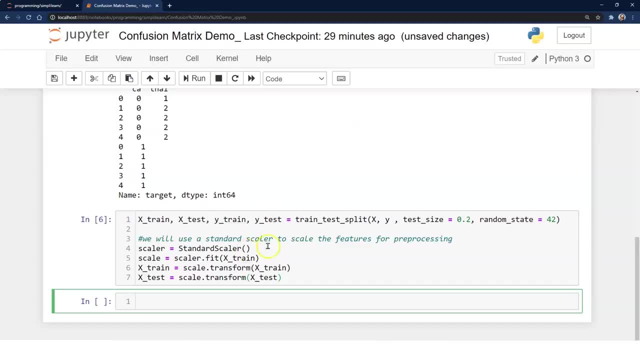 take. here's our X train, X test test, y train, y test. We create our scaler, We go ahead and scale. The scale is going to fit the x train. And then we're going to go ahead and take our x train and transform it, And then we also. 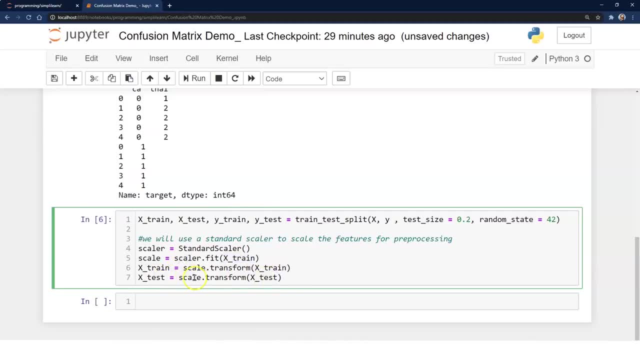 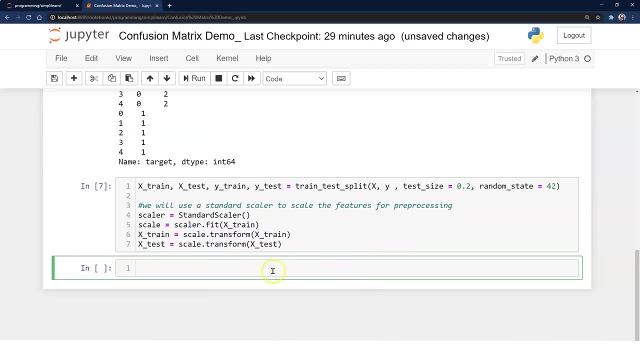 need to take our x test and transform it based on the scale on here so that our x is now between that nice minus one to one. And so this is all our pre-data setup And hopefully all of that looks fairly familiar to you if you've done a number of our other classes and you're up to the setup on. 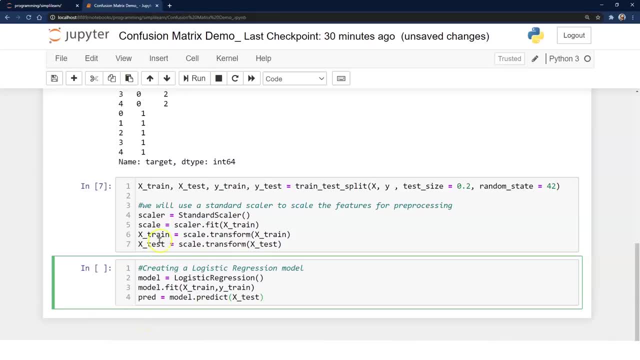 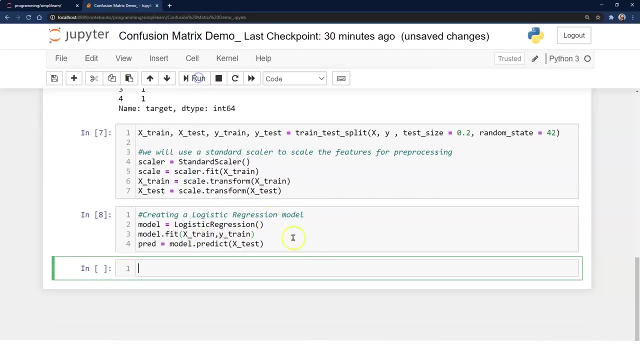 here. And then we want to go ahead and do is create our model And we're going to use a logistic regression model And from the logistic regression model we're going to go ahead and fit our x train and y train And then we'll run our predicted value on here. And so let's go ahead and run that. 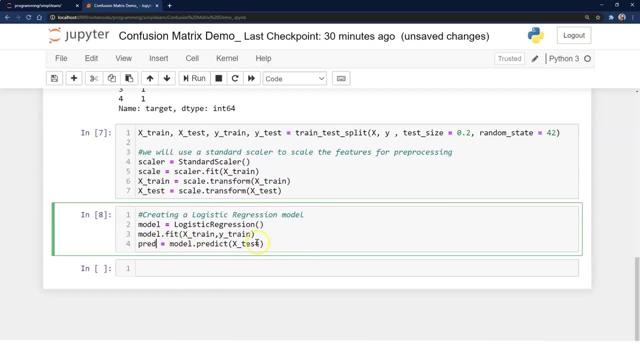 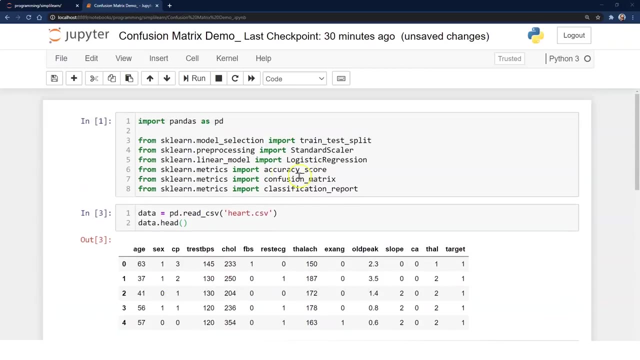 And so now we actually have like our x test and our prediction. So if you remember from our matrix, we're looking for the actual versus the prediction and how those compare. And if I take us back up here, you're going to notice that we imported the accuracy score. 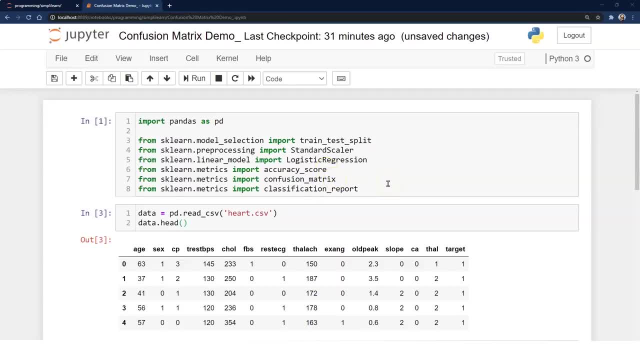 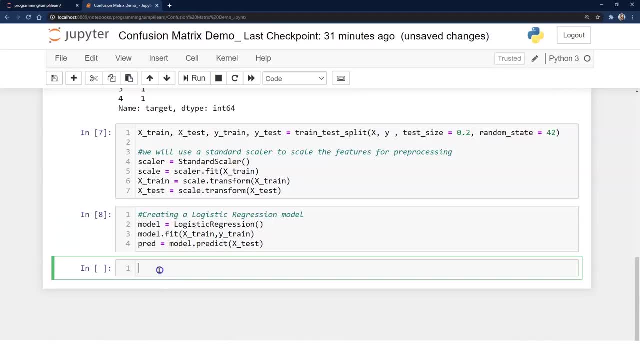 the confusion matrix and the classification report. And there's, of course, our logistic regression, the model we're using for this, And I did mention I was going to talk a little bit about scalar and the regression model, The scalar on a lot of your regression. 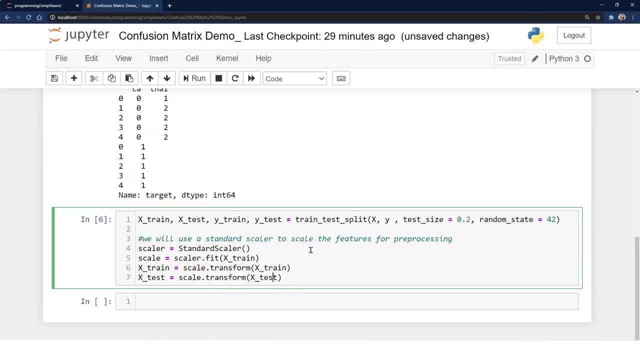 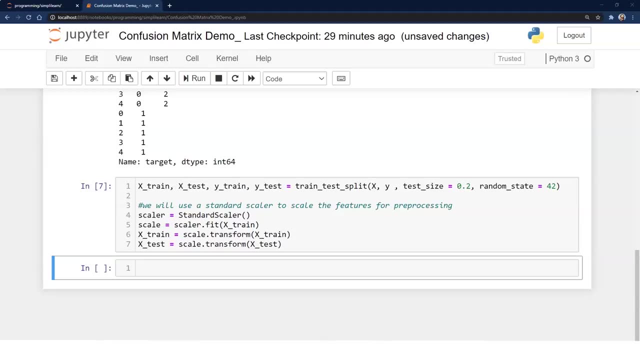 so that our X is now between that nice minus 1 to 1.. And so this is all our pre-data setup And hopefully all of that looks fairly familiar to you if you've done a number of our other classes and you're up to the setup on here. 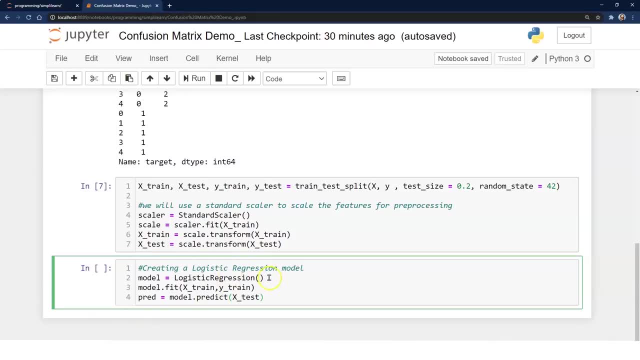 And then we want to go ahead and do is create our model And we're going to use a logistic regression model And from the logistic regression model we're going to go ahead and fit our X train and Y train And then we'll run our predicted value on here. And so let's go ahead and run that. 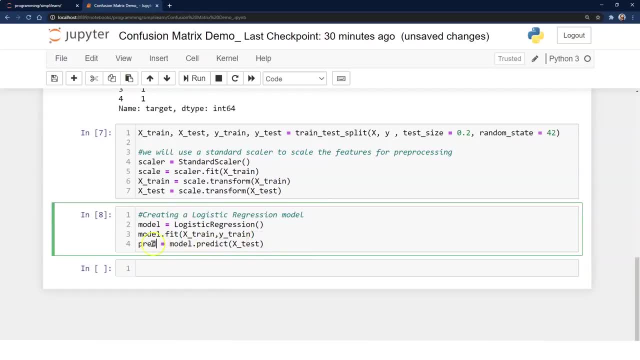 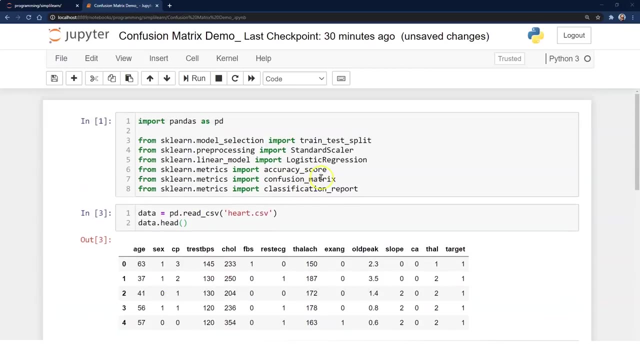 And so now we actually have our X test and our prediction. So if you remember from our matrix we're looking for the actual versus the actual And so we're going to go ahead and the prediction and how those compare. And if I take us back up here, you're going to notice that 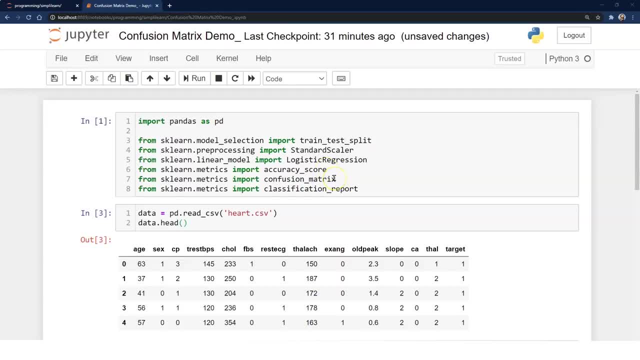 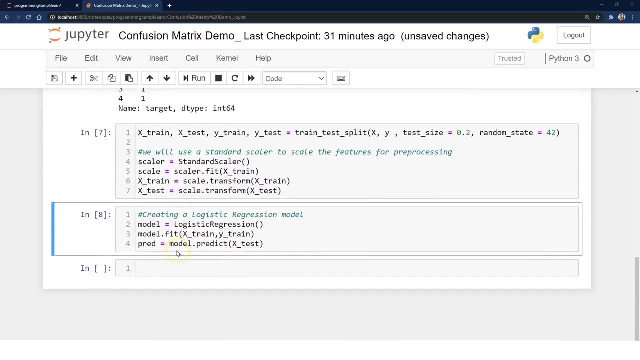 we imported the accuracy score, the confusion matrix and the classification report, And there's, of course, our logistic regression, the model we're using for this, And I did mention I was going to talk a little bit about scalar and the regression model- The scalar- on a lot of your regression. 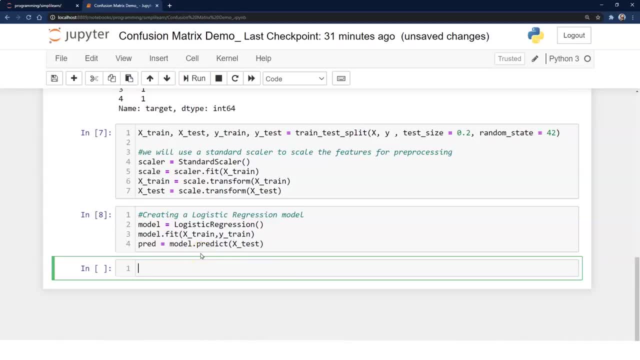 models, your basic mass standard regression models, and I'd have to look it up for the logistic regression model. When you're using a standard regression model, you don't need to scale the data. It's already just built in. by the way, the model works in most cases. But if you're 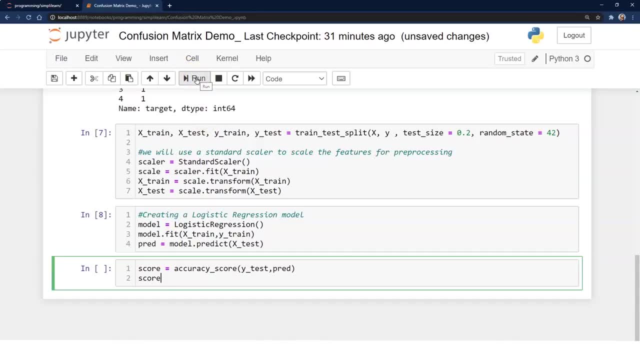 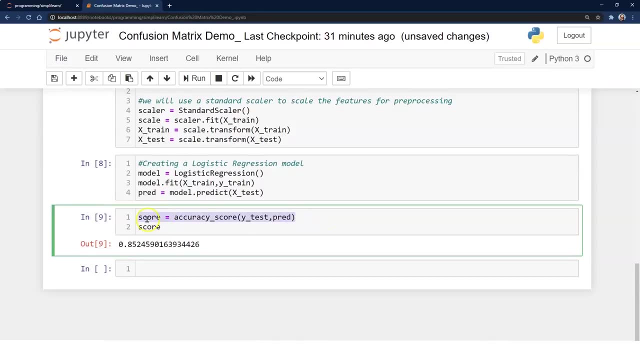 in a neural network and there's a lot of other different setups, then you really want to take this and fit that on there, And so we can go in and do the accuracy. And this is, if you remember correctly, we were looking at the accuracy with the English speaking. So this essentially. 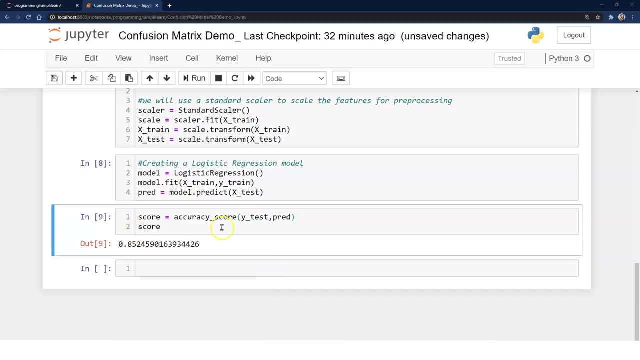 is saying our accuracy as to whether this person is. I believe this is the heart data set. It's going to be accurate about 85% of the time as far as whether it's going to predict the person's going to have a heart condition or the one as it comes up with the zero one on there. 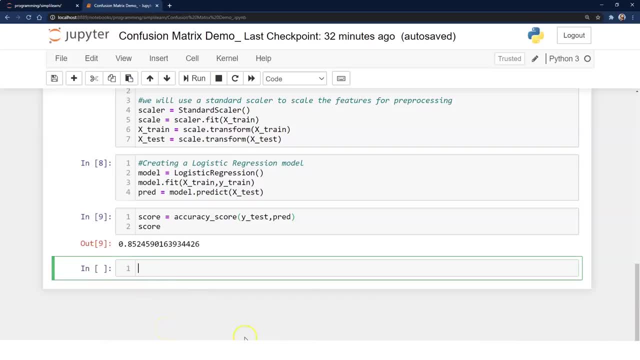 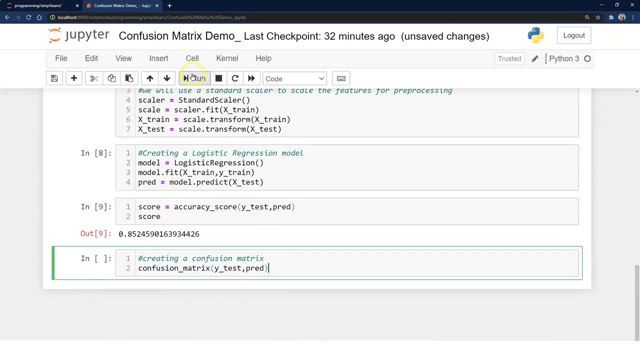 Which would mean at this point that you have an 85% being correct on telling someone they're extremely high risk for a heart attack, kind of thing. So we want to go ahead and create our confusion matrix, And let me just do that. Of course, the software does everything for us, So we'll go ahead and run this. 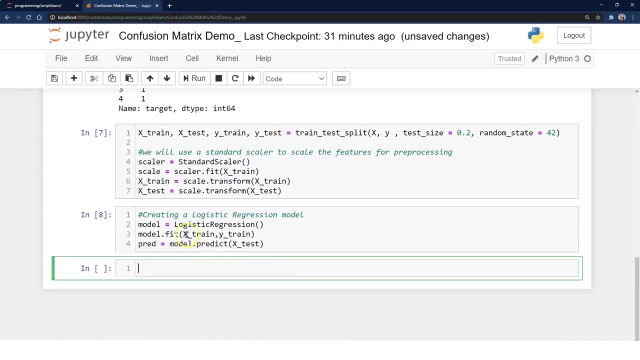 models, your basic mass standard regression models, and I'd have to look it up for the logistic regression model. When you're using a standard regression model, you don't need to scale the data. It's already just built in. by the way, the model works In most cases. but if you're 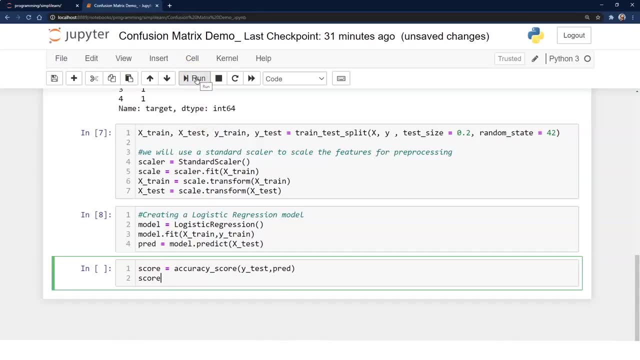 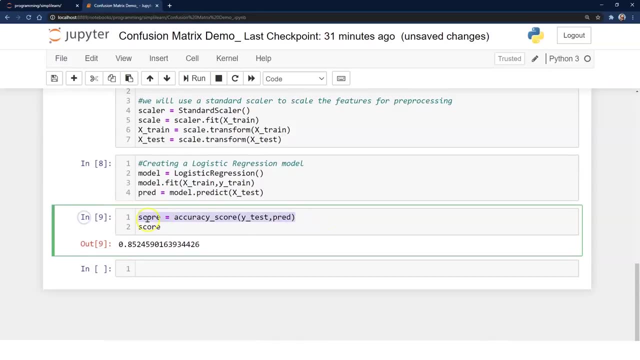 in a neural network and you're there's a lot of other different setups, then you really want to take this and fit that on there, And so we can go in and do the accuracy. And this is, if you remember correctly, we were looking at the accuracy. 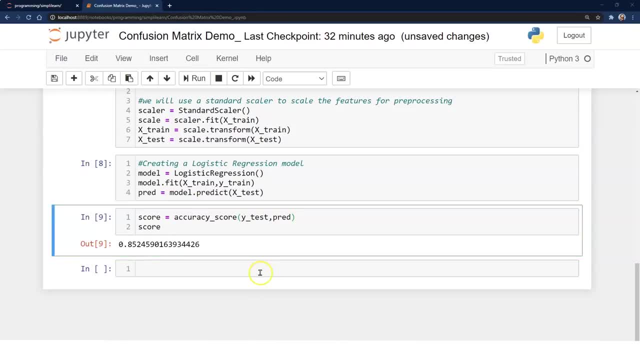 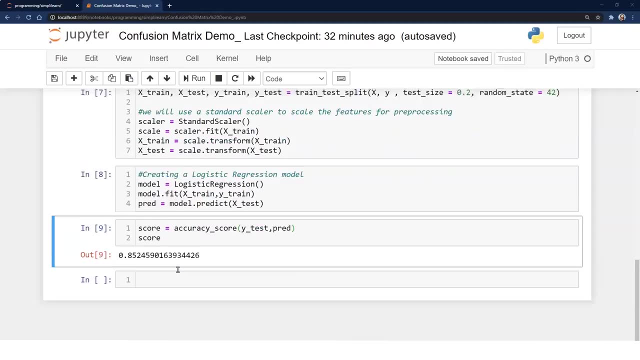 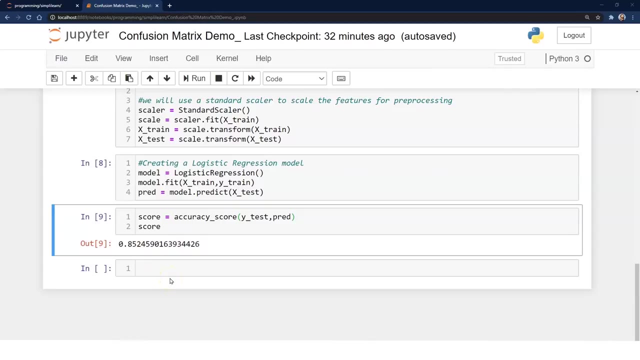 With the English speaking. So this is saying our accuracy as to whether this person is. I believe this is the heart data set. It's going to be accurate about 85% of the time as far as whether it's going to predict the person's going to have a heart condition or the one as it comes up with. 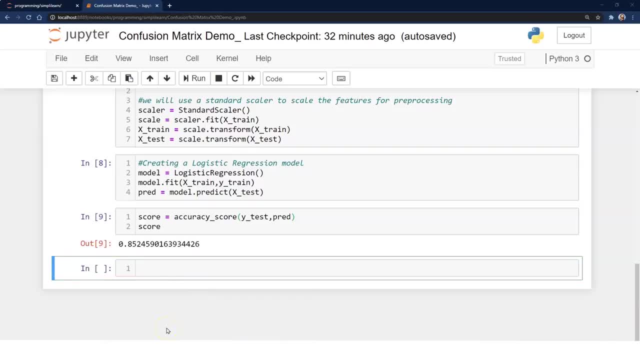 the zero one on there, Which would mean at this point that you have an 85% being correct on them and they're extremely high risk for a heart attack kind of thing. And so we want to go ahead and create our confusion matrix And we just do that. Of course, the software does everything for. 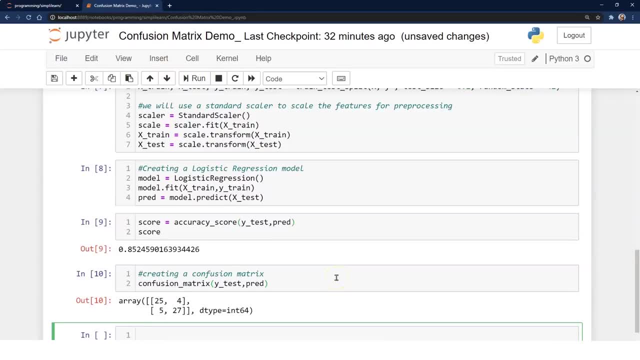 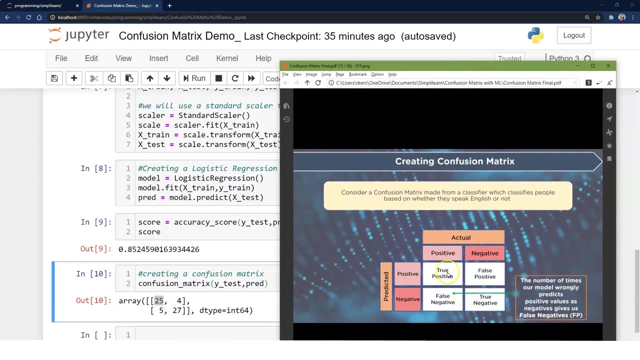 us. So we'll go ahead and run this And you can see right here: Here's our 25 prediction, correct predictions, right here, And if you remember from our slide, just bring this over. So it's a nice visual. We have our true positive, false positive. So we had 25, which were true, that it said. 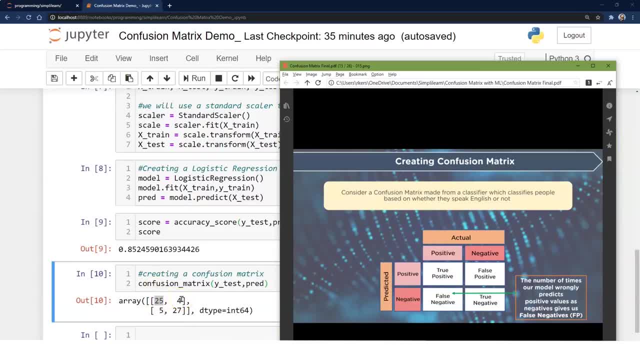 hey, this person's going to be high risk at heart And we had four that were still high risk. that it said were false. So, out of these 25 people, or out of these 29 people- and that makes sense because you have 0.85.. Out of 29 people- it was correct on 25 of them, And so here's our accuracy score. 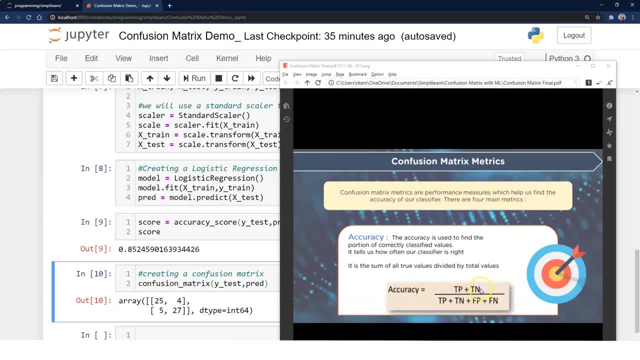 We were just looking at that. Our accuracy is your true positive and your true negative over all of them. So how true is it? And there was our accuracy coming up here: 0.85.. And then we have our nice matrix generated from that And you can. 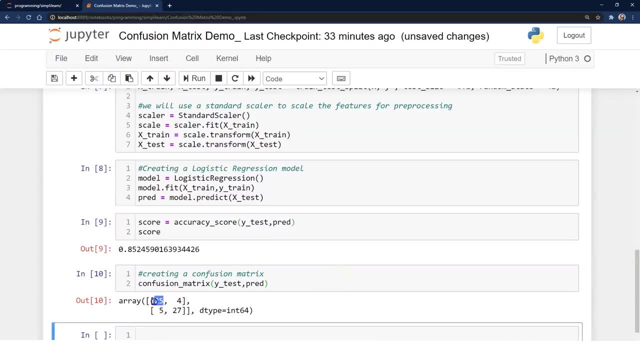 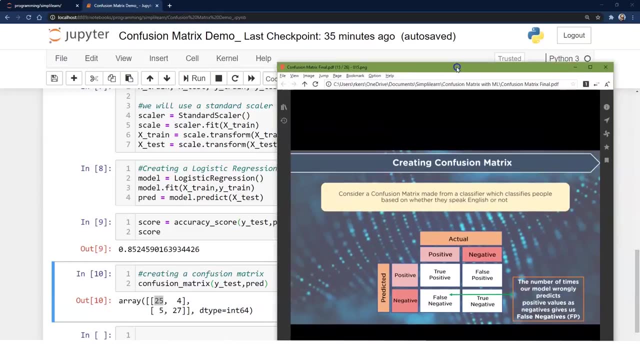 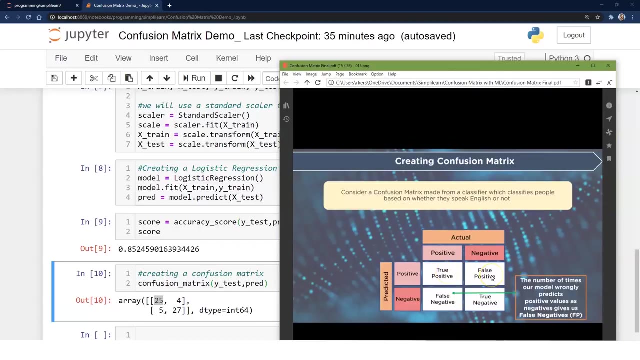 And you can see right here. here's our 25 prediction, correct predictions right here, And if you remember from our slide, I'll just bring this over, so it's a nice visual. We have our true positive, false positive. So we had 25, which were true, that it said: Hey, this person's going to be high risk at heart. 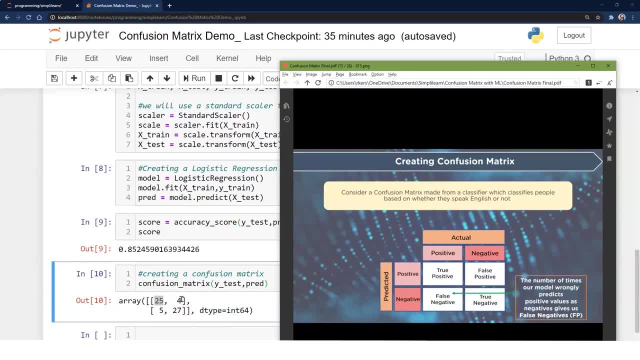 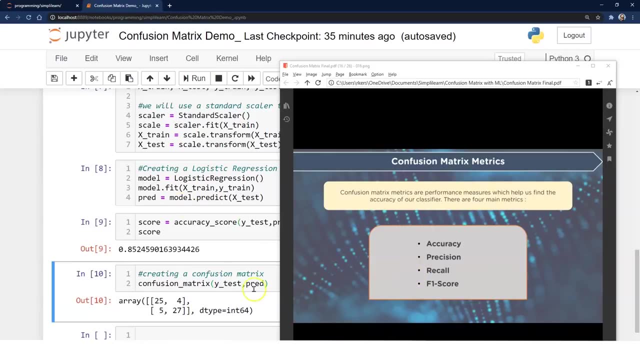 And we had four that were still high risk, that it said were false. So, out of these 25 people, or out of these 29 people- and that makes sense because you have 0.85 out of 29 people- it was correct on 25 of them, And so here's our accuracy score. We were just 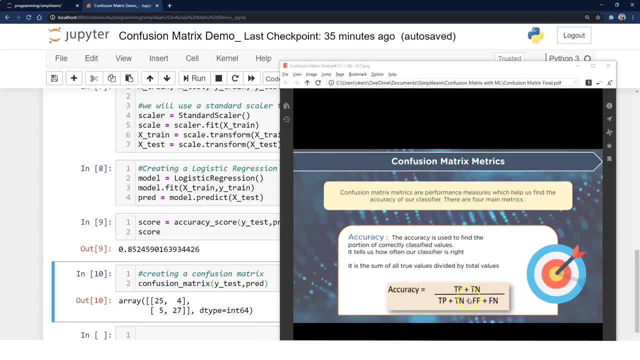 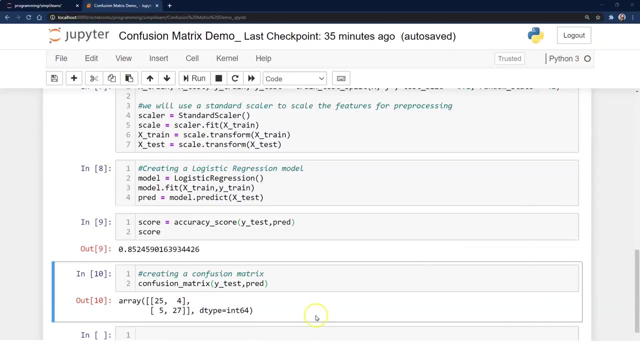 looking at that. Our accuracy is your true positive and your true negative over all of them. So how true is it? there was our accuracy coming up here 0.85. and then we have our nice matrix generated from that and you can see right here is a similar matrix. we had going for that from the slide and this starts. 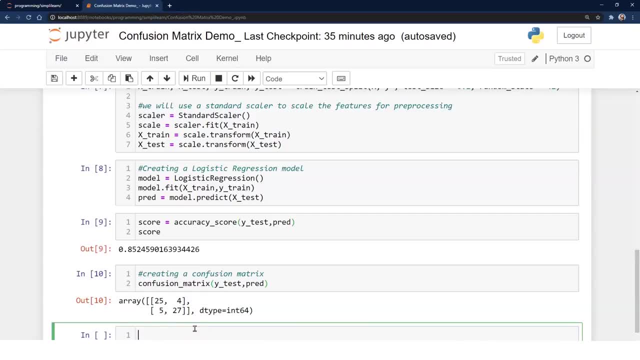 to this should start asking questions at this point. so if you're in a board meeting or you're working with this, you really want to start looking at this data here and saying, well, is this good enough, is this number of people? and hopefully you'd have a much larger data set. 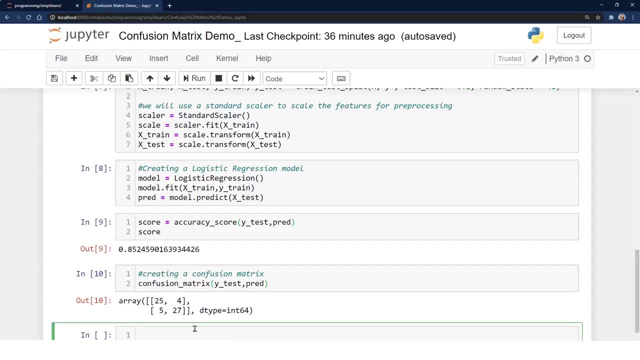 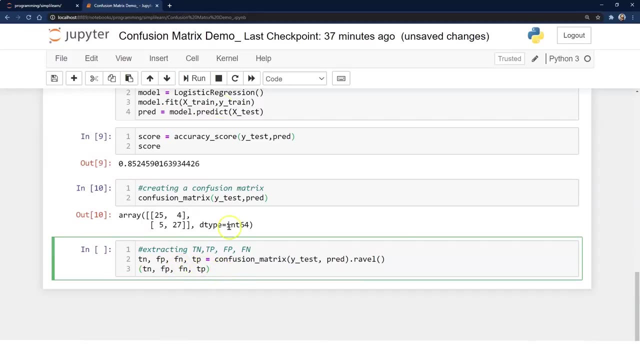 it might. is my confusion matrix showing for the true positive and false positive. is that acceptable for what we're doing? and, of course, if you're going to put together whatever data you're putting out, you might want to separate the true negative, false positive, false negative- true positive, and you can simply do that by doing the confusion matrix. and then, of course, the ravel. 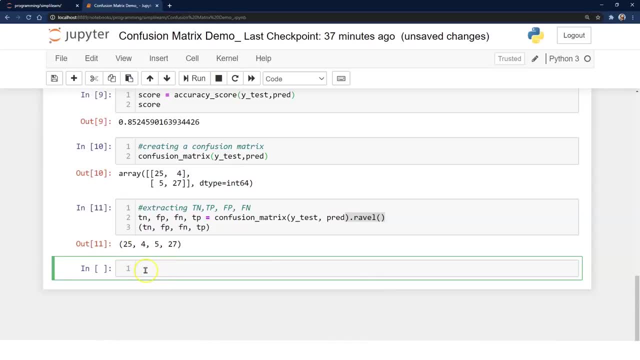 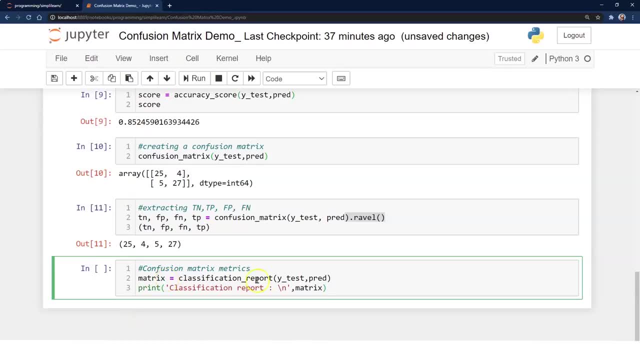 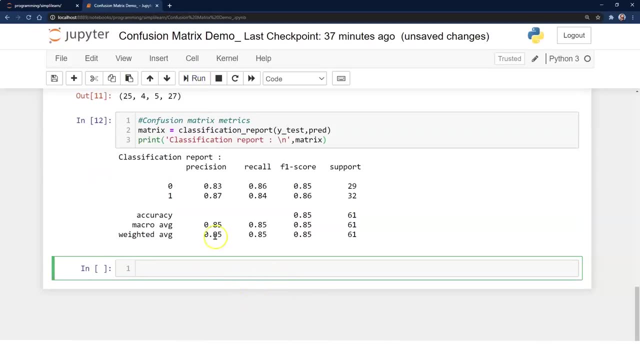 come in here and just use the matrix equals classification report, the y test and the predict, and then we're going to take that classification report and go ahead and print that out and you can see here it does a nice job, giving you your accuracy, your micro average, your weighted 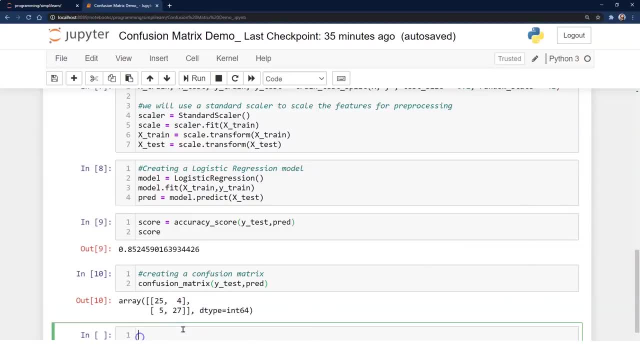 see right. here is a similar matrix. we had going for that from the slide, And this should start asking questions at this point. So if you're in a board meeting or you're working with this, you really want to start looking at this data here and saying, well, is this good enough, Is this number? 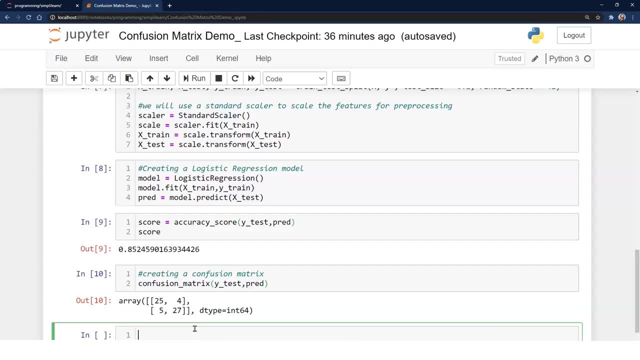 of people being used correctly And hopefully you'd have a much larger data set. Is my confusion: matrix showing for the true positive and false positive? is that acceptable for what we're doing? And, of course, if you're going to put together whatever data you're putting out, you might want to separate the 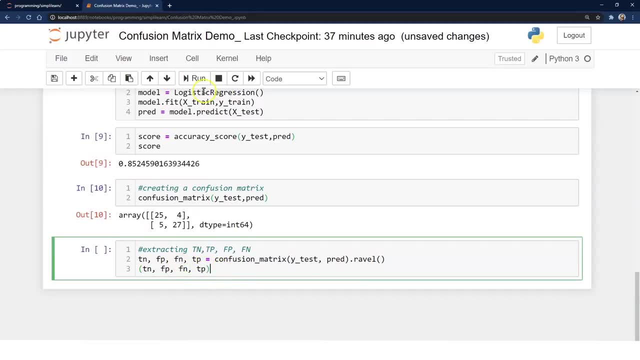 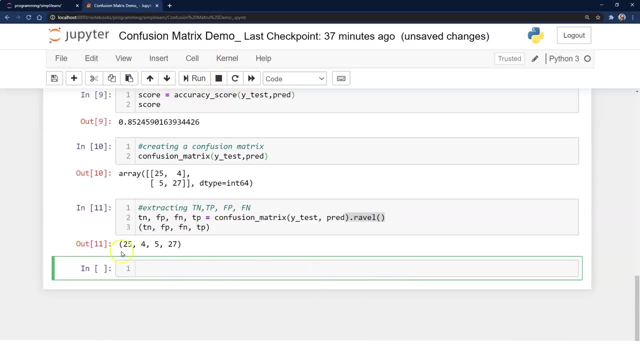 true, negative, false positive, false negative, true positive. And you can simply do that by doing the confusion matrix. And then of course, the ravel part lets you set that up, So you can just split that right up into a nice tuple. 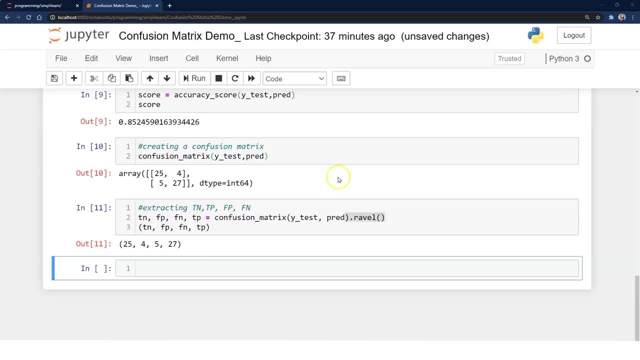 And the final thing we want to show you here in the coding on this part is the confusion: matrix metrics. And so we can come in here and just use the matrix equals classification report, the Y test and the predict, And then we're going to take that classification report and go ahead and print that out. 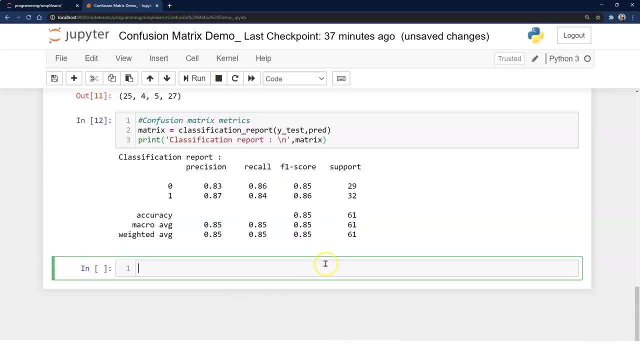 And you can see here it does a nice job, giving you your accuracy, your micro average, your weighted average. you have your precision, your recall, your F1 score and your support all in one window. So you can start looking at this data and saying, oh okay, our precision's at 0.83, 0.87 for getting a positive and 0.83 for the negative side for a zero. 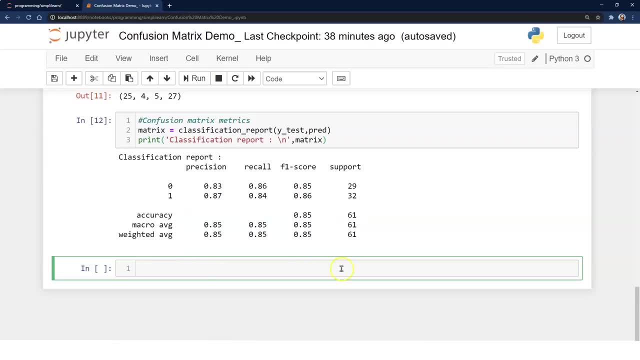 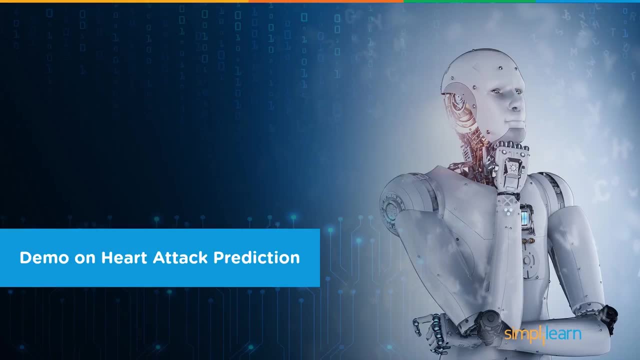 And we start talking. And we start talking about whether this is a valid information or not to use. And when we're looking at a heart attack prediction, we're only looking at one aspect: What's the chances of this person having a heart attack or not? 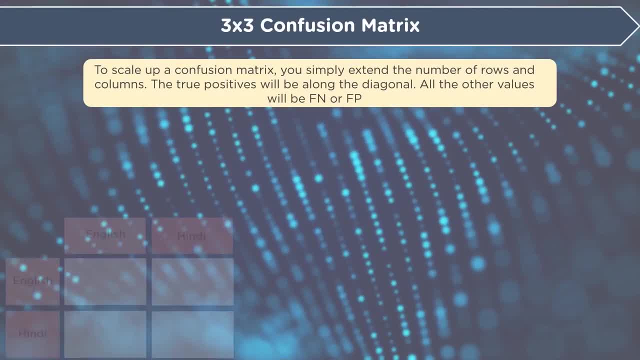 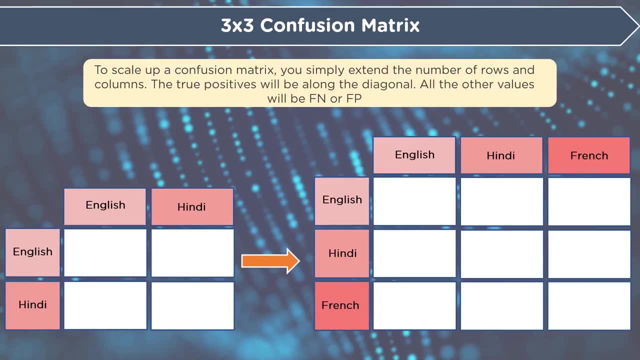 You might have something where we went back to the languages. Maybe you also want to know whether they speak English or Hindi or French, And you can see right here that we can now take our confusion matrix and just expand it as big as we need to. 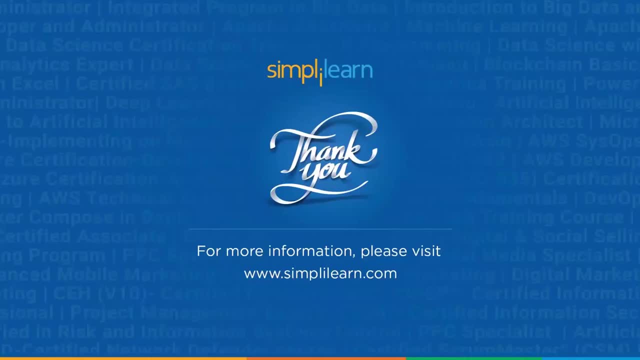 depending on how many different classifiers we're working with. So thank you for joining us today. For more information, please visit wwwsimplylearncom. Get certified, get ahead.